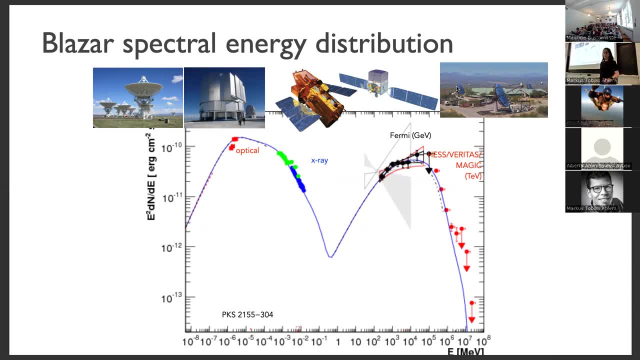 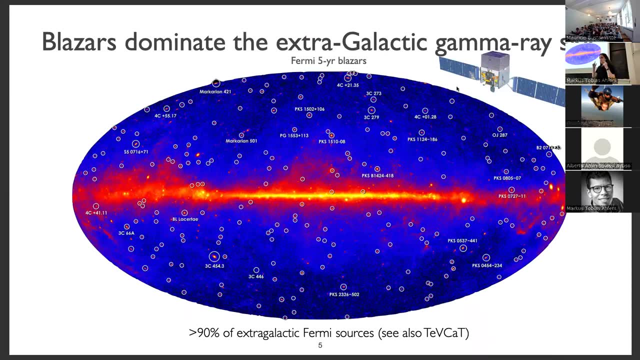 thought this is probably inverse coupton emission from those same electrons And it goes all the way up to TV energies and some lasers, So very high energy gamma rays. And this was also also our motivation. why blazers were chosen for this? because they absolutely dominate. 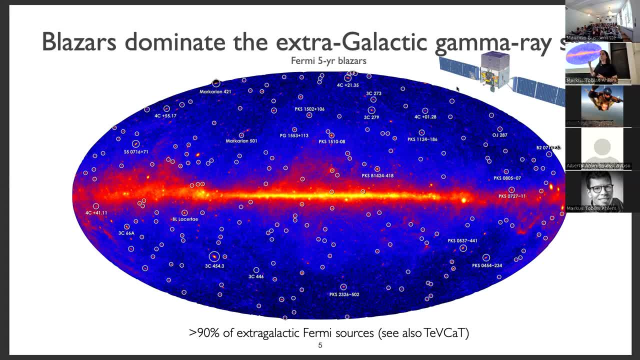 the extragalactic gamma ray sky, So they are the overwhelming majority of TV and GV gamma ray sources that we know from outside our own galaxy. This means for sure they accelerate particles to very high energies, And the question that we're going to work through today is: 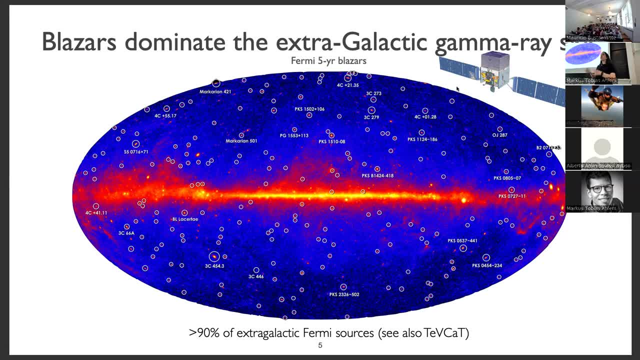 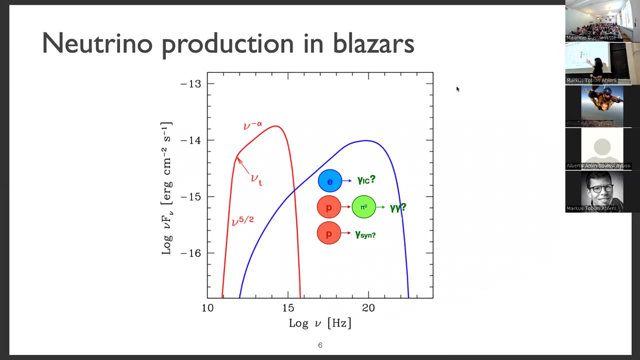 do they only accelerate electrons Or do they also accelerate protons? Because gamma rays might be just produced by electrons, but then we don't get neutrinos. So yeah, as I was saying before, previously we worked with this model in which the all the gamma rays 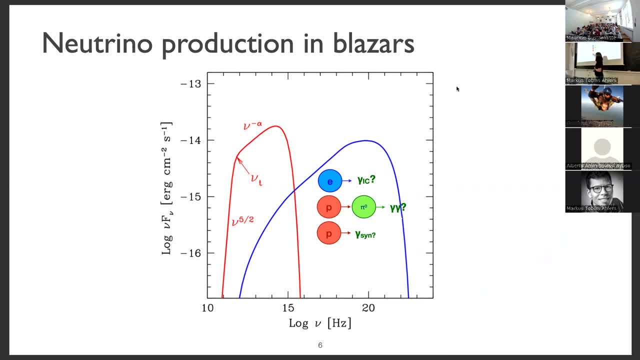 come from electrons And, you know, up scattering these photons or other photons close to the black hole. but it could well be this shape of gamma rays that we see could well be produced by neutral pions decaying to gamma rays, And or it could. 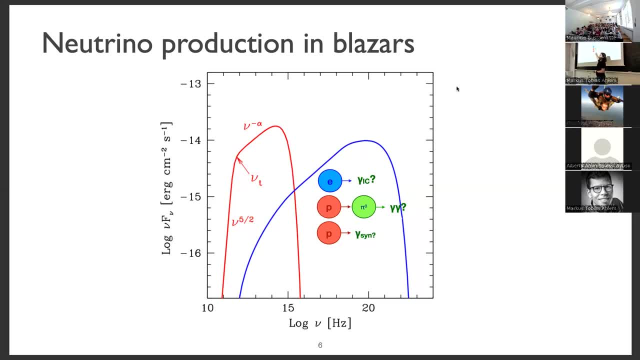 be proton synchrotron emission producing these gamma rays. So there are several possibilities for this origin of this gamma ray emission And in this case in particular, but also in the proton synchrotron case, we will get neutrinos in addition from this blazer And it's reasonable. 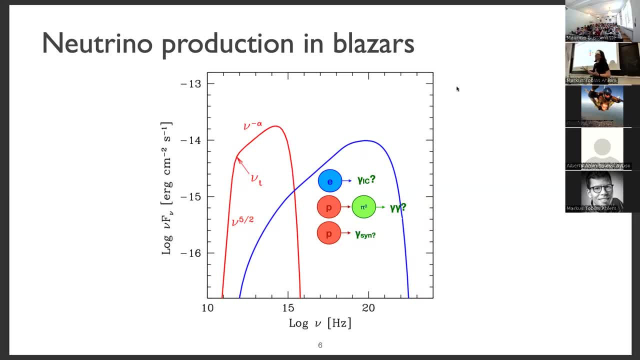 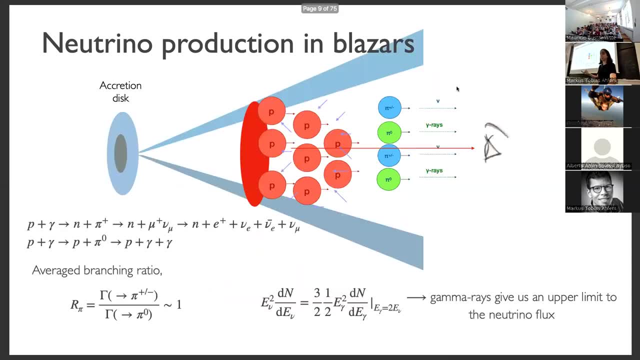 that some high energy protons are there in this jet. The question is really how many and what energies they reach, and so on. This is what matters for neutrino production. So sort of schematic of what's happening in this, in this, in this source. So we have in. 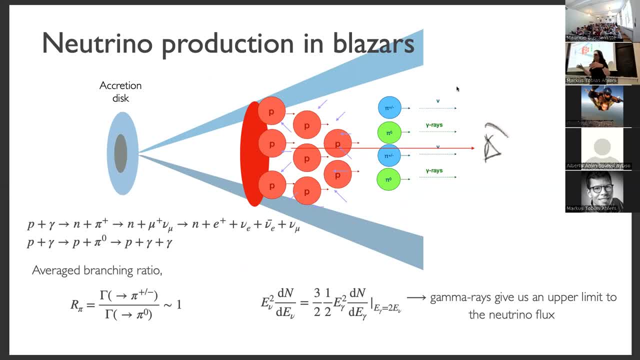 the blazer jet. we have many options where we can have a shock, where we can accelerate protons. maybe there is a long lift standing shock, or maybe there are many shocks being formed as matter. plasma goes at these relativistic speeds down the jet. 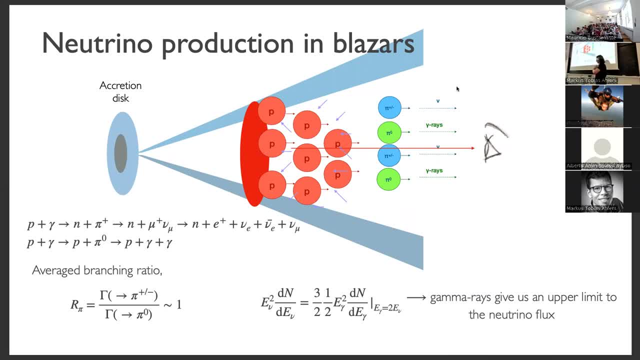 And so these protons are somewhere relativistically traveling down the jet and they have photopion interactions with photons, Either from the jet itself- we've seen these jets, right, they're very bright- So either photos in the jet or there are photons associated with the black hole, with the supermassive 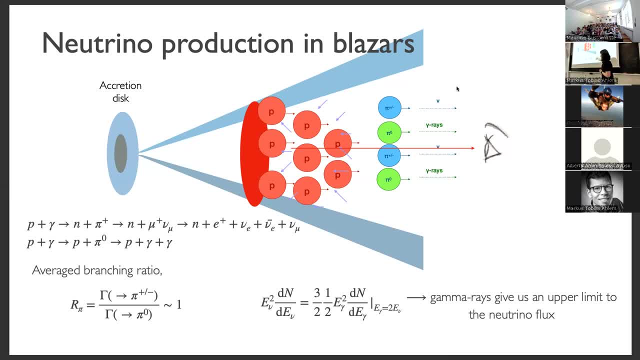 black hole And in these interactions we get. you know, the branching ratio for neutral or charged ions is the same. roughly that means we get: for every three neutrinos we get two gamma rays. So the gamma rays have each half the energy of the pion, The neutrinos have each a quarter. 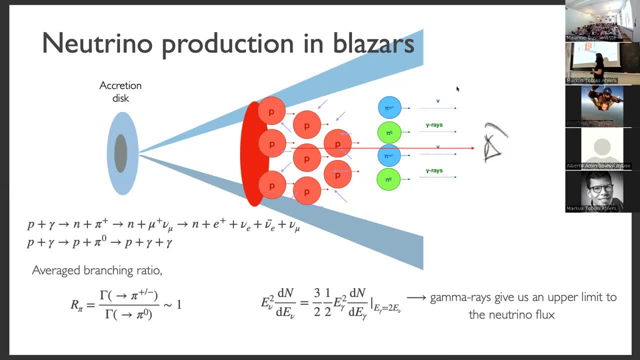 of the energy of the charged pion. Therefore, each neutrino has half the energy of each gamma. So here I've written, So I've written the relation. okay, we have three neutrinos for every two gamma rays. So these are these factors here, and except for this, which is roughly 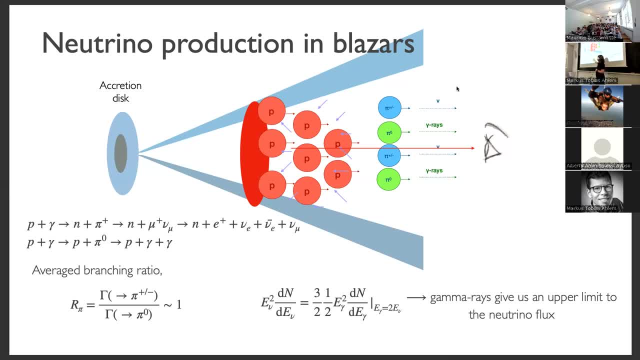 one, the energy flux of neutrinos equals the energy flux of gamma rays in photobiome interactions. so this is a useful thing to remember: that every time you see a gamma ray flux in any kind of source, that gives you an upper limit to the neutrino flux in that source. and why do i say upper limit? because gamma rays can come from other. 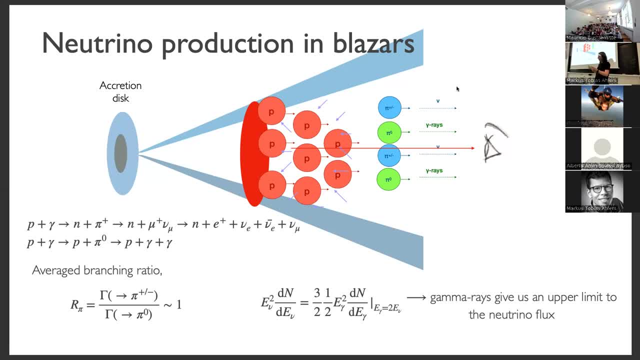 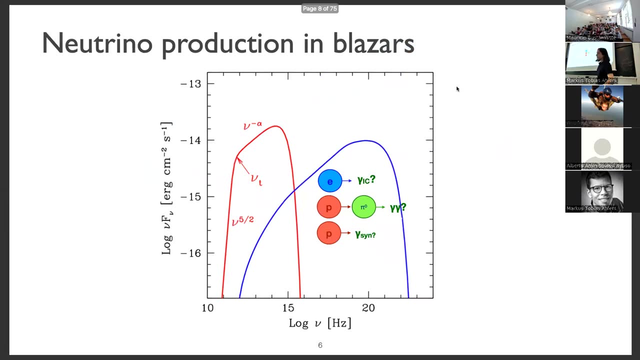 leptonic processes. so electron emission, but neutrinos have to be associated with gamma ray production because of this branching ratio. so if we, if we were to go back to this source, we could say that the neutrino flux can be at most this much. okay, is this clear to everyone? 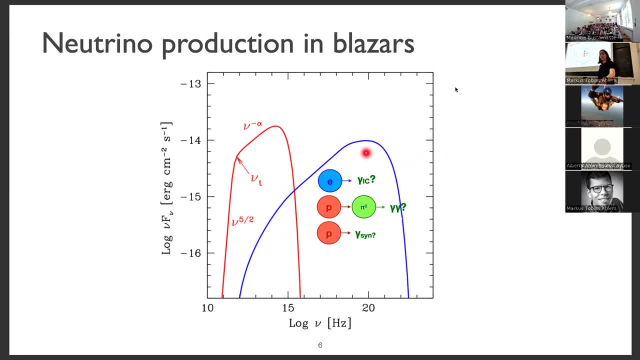 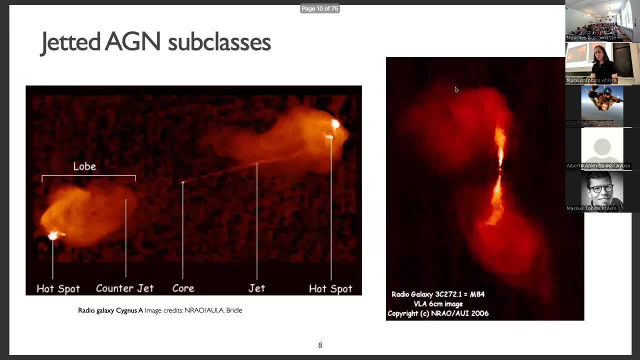 because these are the gamma rays here, and we we just said that there should have the same normalization at most. so just to remind you that when we look at the data, we can see that there are two classifications actually. now there is a third one for even weaker. 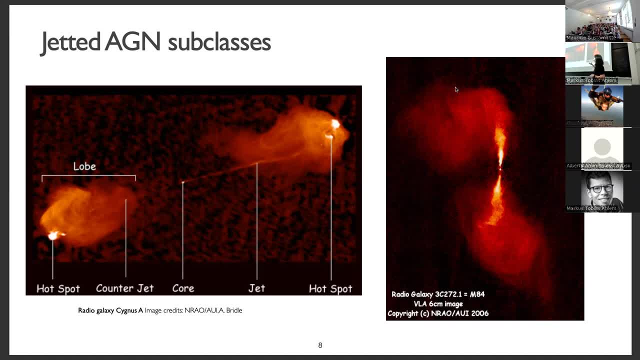 jets. that doesn't matter so much. but these very powerful jets are associated with very efficient accretion close to the eddington limit, and we said that the unification model describes all agn based on few parameters. that is, when we look at the very powerful blazar this is, we don't know what. 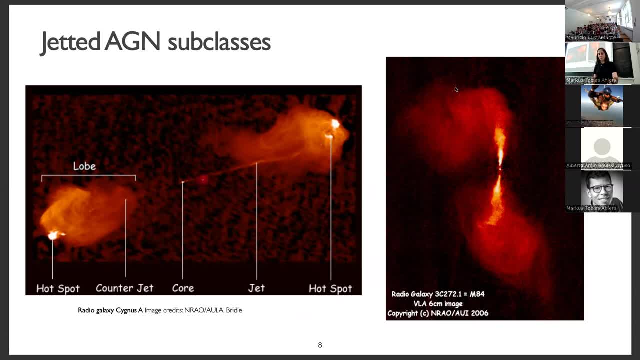 it's going to look like, but we can see that it's going to look like this. we can see that it's going to look like this, but we know it is of this type, if this unification model is perfectly correct, of this very, uh, collimated powerful. do you have a question? okay, powerful, uh jets. 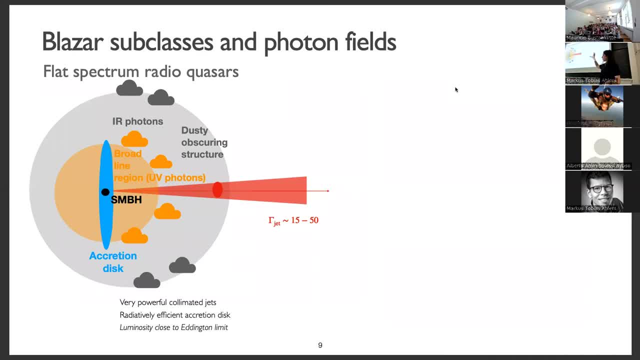 and so in this case, of that powerful type, collimated, what we call fr2 radio galaxies, we have a lot of photons related to the accretion disk, we have dust and this is the emission lines. so on wednesday, these broad emission lines, they reveal the presence of hot ionized gas surrounding 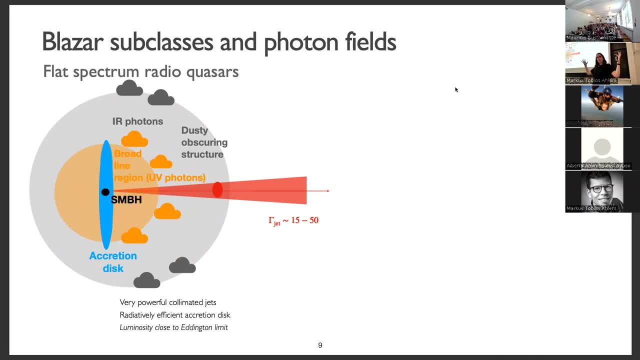 the black hole. and in addition, there was this dust torus that we saw in one photo that also intercepts and re-radiates the light from the, from the, from the disk to infrared. so these are great, because for neutrino production we need a target medium, and these are our target medium. now, if we 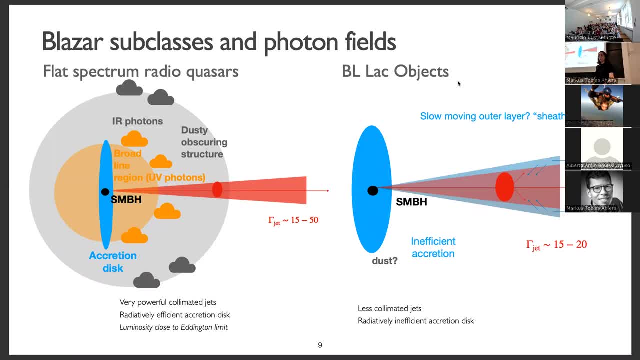 have this other laser material, then we will only have one electron. so let's say you have a high tolerance of light. then we also have the same randomization law. so if we have a received in someone we can say plus or minus zero. so you can say plus or minus zero. so it's. 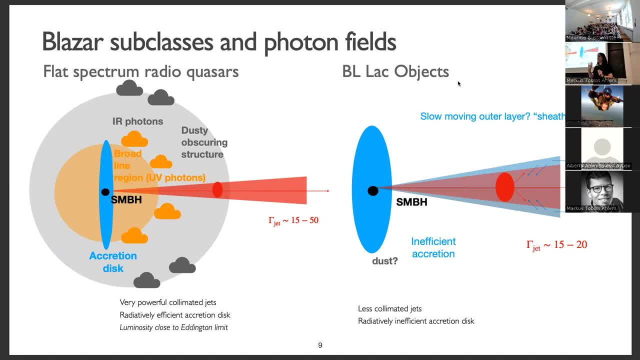 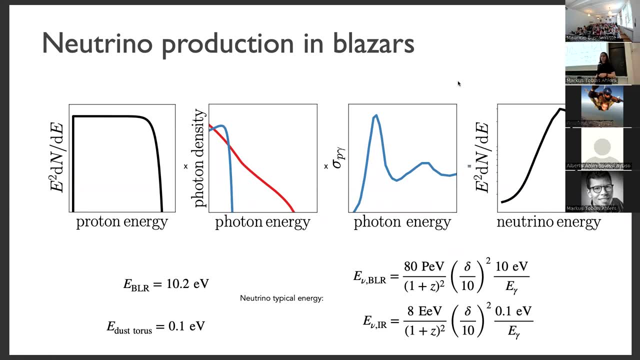 just you can say plus or minus zero and then you can set the furthest distance. so on the left side you can see a flash that will give us this idea of about the input current and you can check it out. if the light is, you can see the. 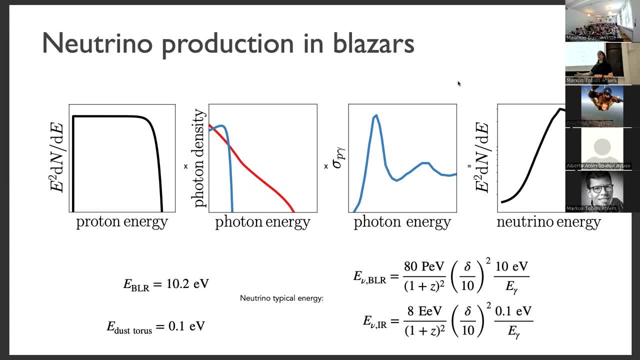 light on the left side. the first light is the energy from the hustler's end, so that's five protons with an e to the minus two spectrum. in terms of the number, that means in terms of the energy flux of the protons, we have this kind of what looks like a straight line, because i've 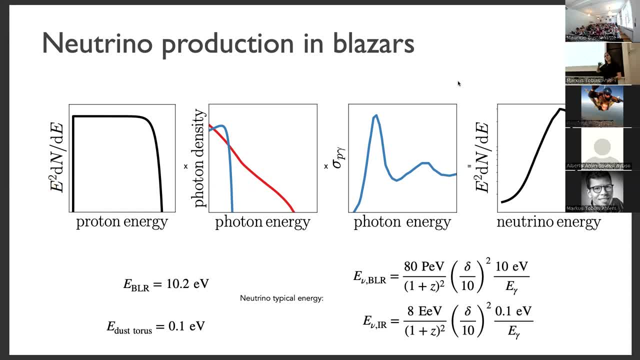 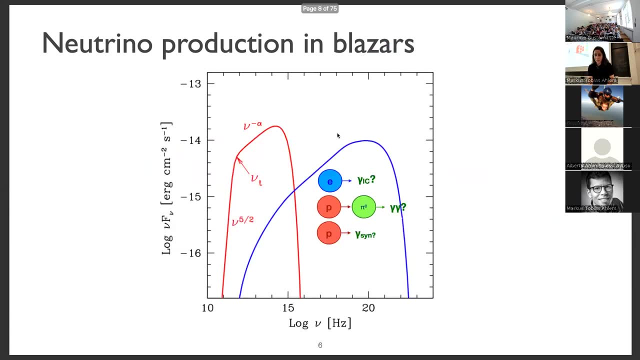 multiplied here by e squared. and so when we have such an e to the minus two power law of protons, what matters for neutrino production is what kind of photon fields these protons are interacting with. okay, now, this is basically this blazer or a similar one. this is energy flux here. sorry that i. 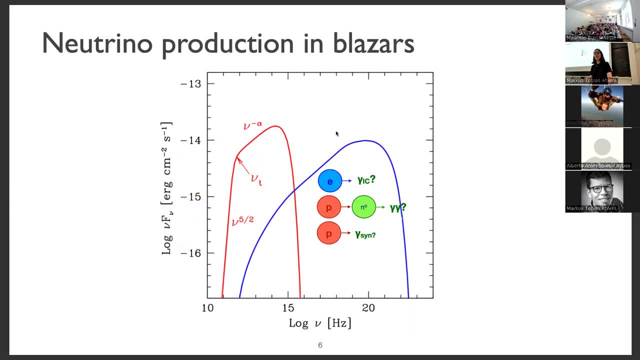 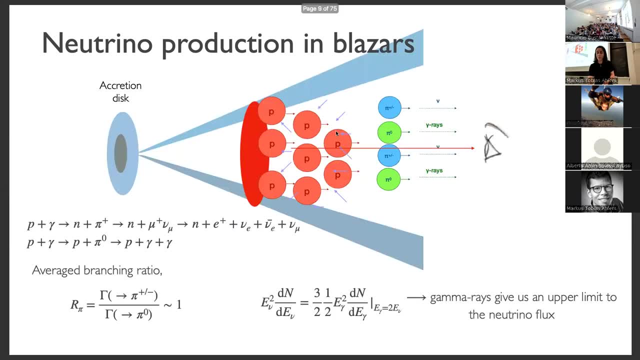 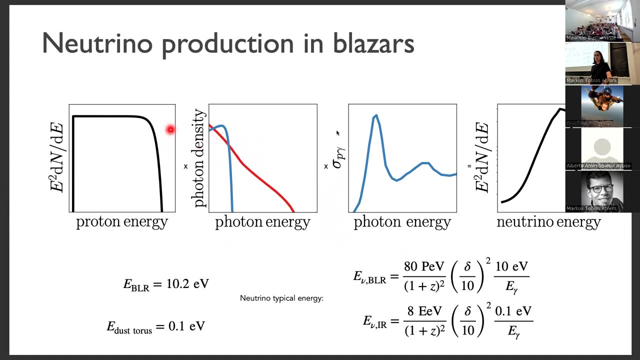 have this. this is astronomy. i should have changed anyway. this is also e squared d and d e, so energy flux, the number flux, is what we saw in the other lot here. so there are way more low energy photons than there are high energy photons and this determines: 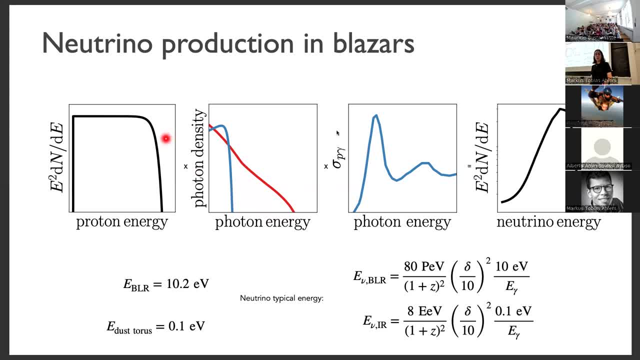 the shape of the neutrino spectrum, because the only the high energy photons have access to these very numerous low energy protons. okay, so otherwise they just don't. they're not, uh, yet at the threshold for pion production and also the for the pion cross-section is resonant, so it's not flat. 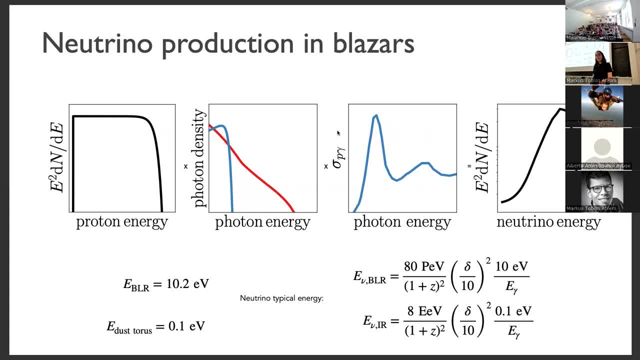 like in proton proton interactions. so, as a result, even though we started off with a proton power law, which is a flat in energy flux, we always get this very geeky spectrum from photopion interactions. so this is true not only for blazers, this is true for photopion interactions. 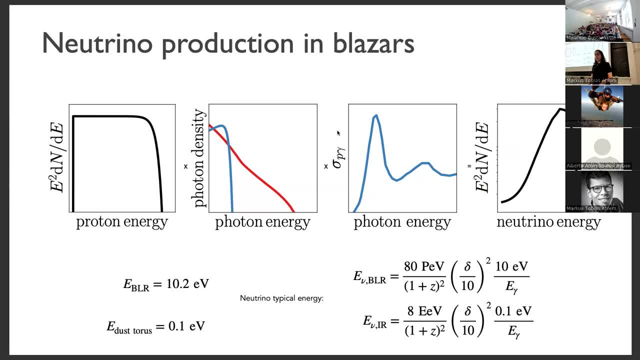 in general, and so all the models that you're ever going to see for blazers have this shape and you can maybe already understand that mark that this doesn't really look like the ice cube neutrino spectrum which is flat over quite a large energy range. But okay, we'll see. I mean, we haven't yet discussed how a whole population 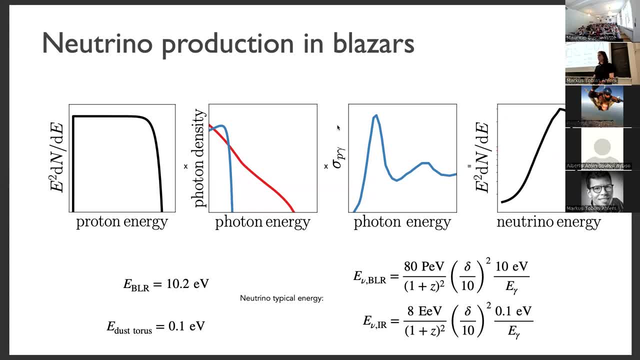 might look like. This is just a single blazer neutrino spectrum. So in addition, just from a simple kinematics calculation we can work out where the peak of the neutrinos spectrum should be. And that's because we understand rather well that all AGN that have an accretion disk 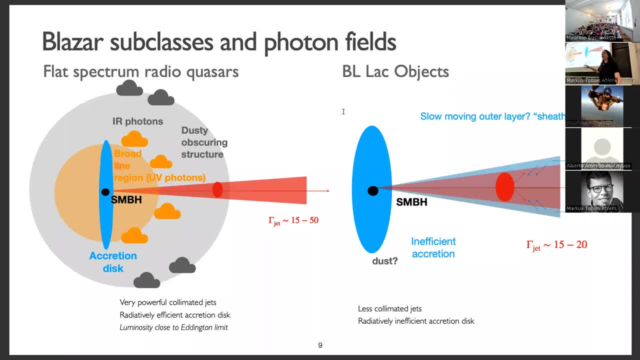 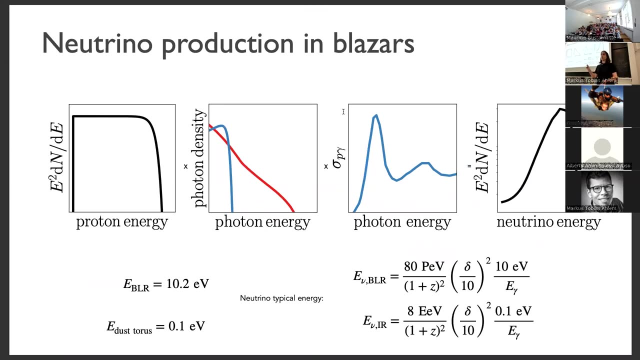 for example, they all have a bump in the UV energy range. So we know that all AGN have this very characteristic photon field with this very specific energy, And so therefore we can always work out what should be the peak of the neutrino flux. So, in the case that this happens, 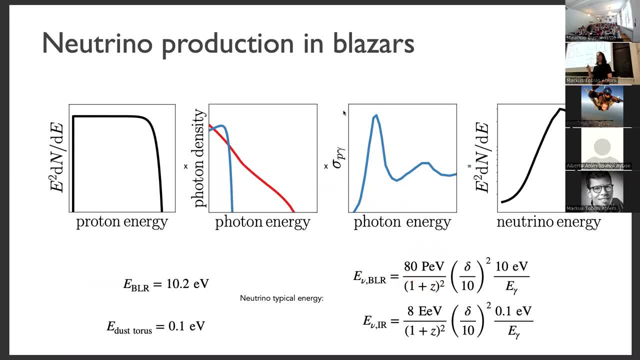 in interactions of high energy protons with UV photons from the accretion disk, then we expect of order tens of keV. That's where the neutrino spectrum should peak. Now, if the interactions are happening with the infrared photons which are down here at low energies, then we have 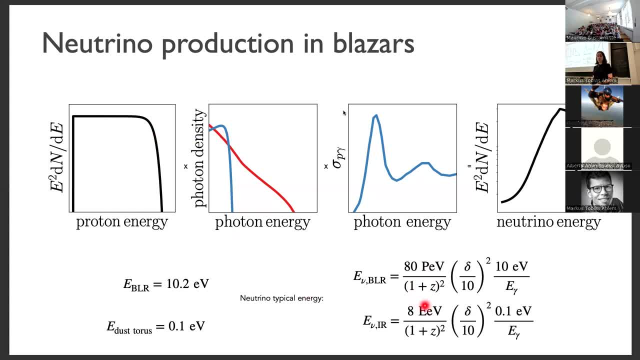 neutrino production at higher energies, at about 10 to the 18 electron volts. This is also true in GRBs- we're going to see in a moment. So we also know where, where the neutrinos should be in energy. So theory tells us already quite a lot about. 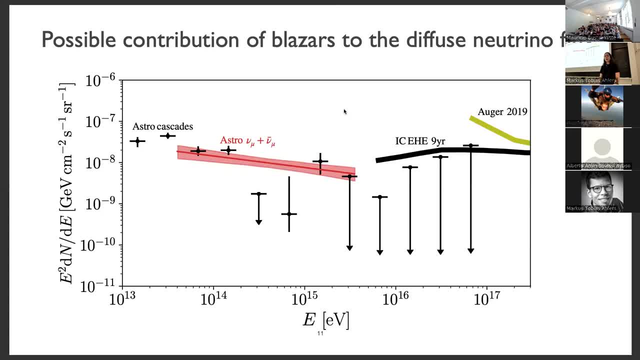 this neutrino spectrum. So now here I have the IceCube data, So you recognize maybe here these are the muon data. So from all the tracks and then the cascades are the black data points, And at high energies, oops, at very high energies, IceCube has not detected any neutrinos. but 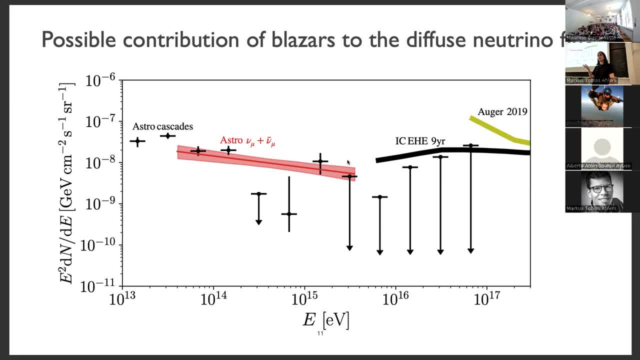 well, that has allowed IceCube to place an upper limit to the total flux from all, from all sources. So we have an upper limit, which is this black line here. And so now, if we look at several blazer models where someone has integrated what I was describing, 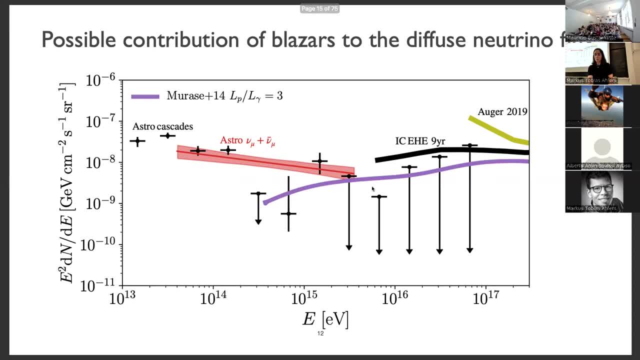 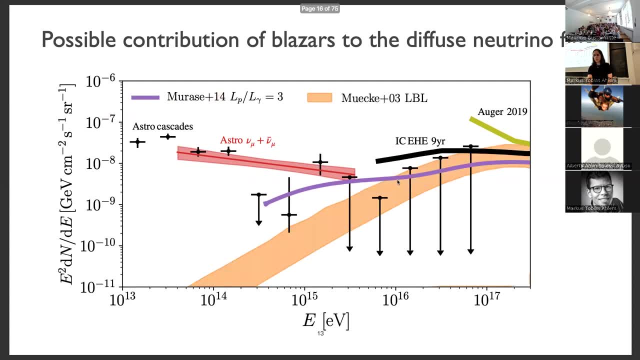 before over the entire population. here is one. it peaks at about 10 to the 18 electron volts. This model was made in 2014.. Another one, made in 2003, also peaks at about 10 to the 18 electron volts, And another one. 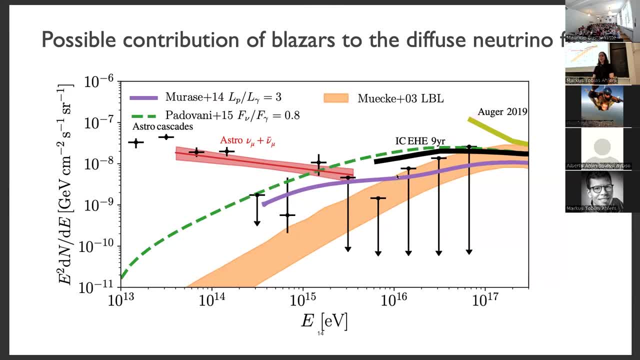 made in 2015,. also the same. So you can already maybe notice that none of these are very good fits to IceCube neutrinos. And you are laughing. you are young and you don't have a prior, But when I say this in a conference with old people, they get very upset. 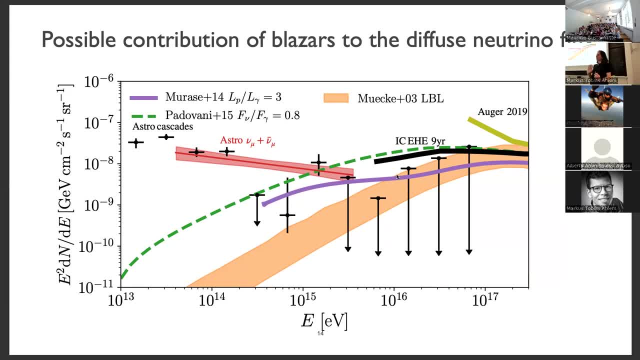 You know, this is the first time I ever heard about it, But I don't want to mess this up, because everybody thought you know, or not everybody, but maybe people think blazers are fantastic, so we should see their neutrinos. but anyway, 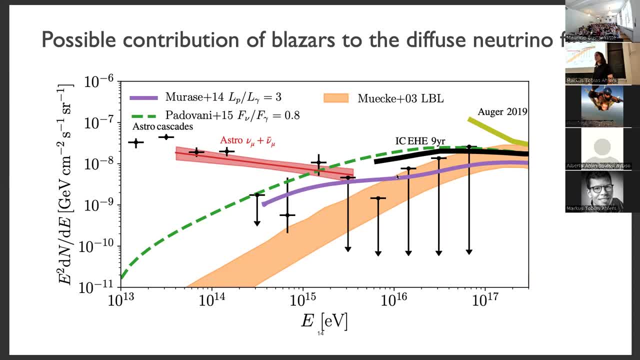 This is a problem, Okay, so theoretically, we expect the blazer neutrino flux to peak at ultra high energies, and this is not what IceCube sees. Now, of course, if the maximum energy is low, what's going to happen is we're going to have a cut off here. So, but still. 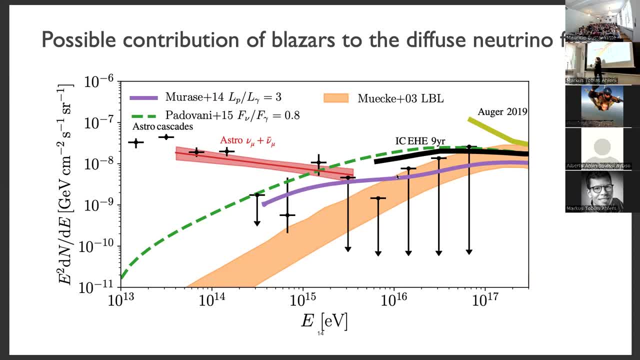 we cannot do anything to push the entire model to the left. So we can get rid of the high energy flux by saying there are no high energy protons but there's nothing. we can do, almost nothing we can do theoretically to change that. 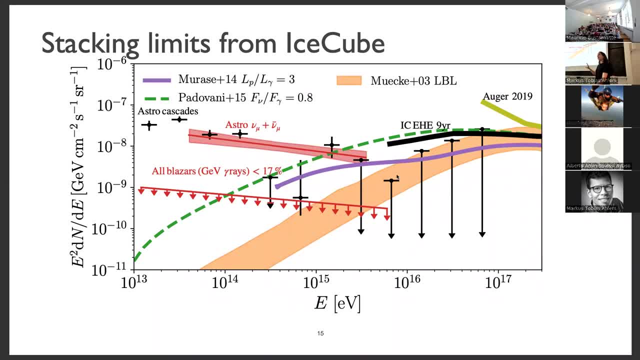 In addition. so IceCube has done, and I'm gonna talk about this throughout the lecture today. IceCube scientists do stacking analysis. This means they take all the known directions of all blazers and they look at whether there is an excess of neutrinos in the directions of those blazers. 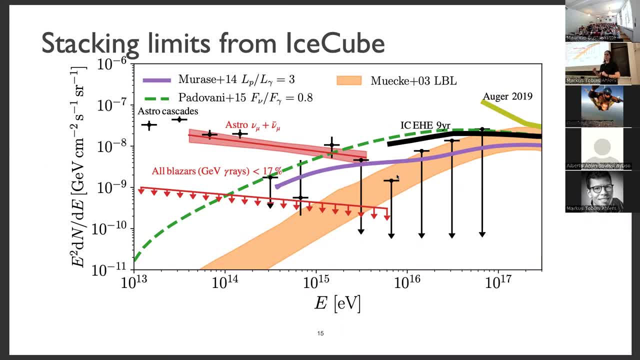 And they do the same for GRBs and everything, And we'll go through this today. So here, this line shows the results of an analysis in which someone looked at all the directions of known gamma ray emitting blazers- about the thousand of them in the catalog. 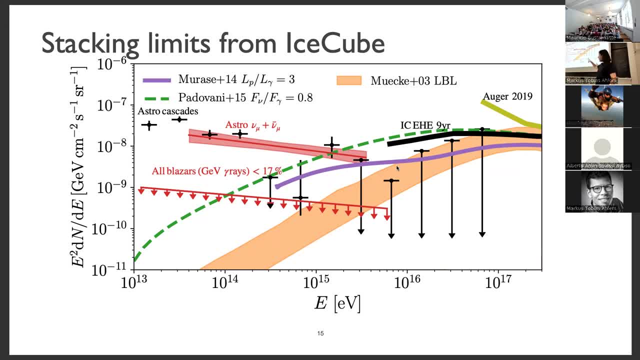 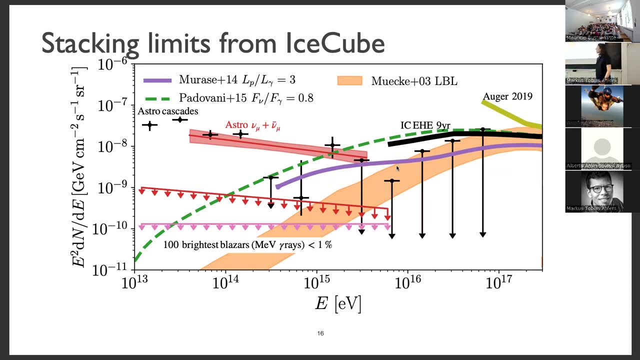 and found no excess. So they were able to place a limit of the order of 20% to the total contribution of blazers to the IceCube neutrino flux. And yesterday there was a new paper on the archive in which they took a different catalog. 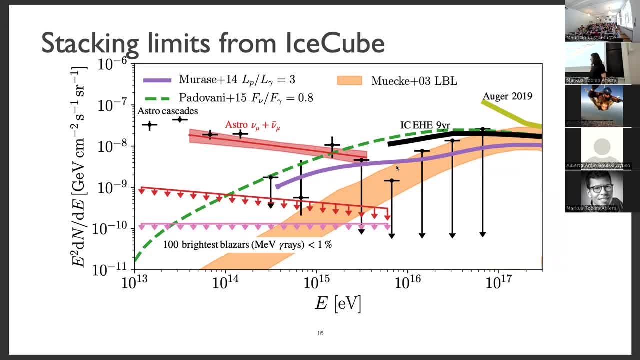 and they took really a hundred brightest blazers, the most luminous blazers, or rather I should say no, they're really just the brightest at Earth. They peak at a slightly different energy And that's actually okay. I don't want to go. 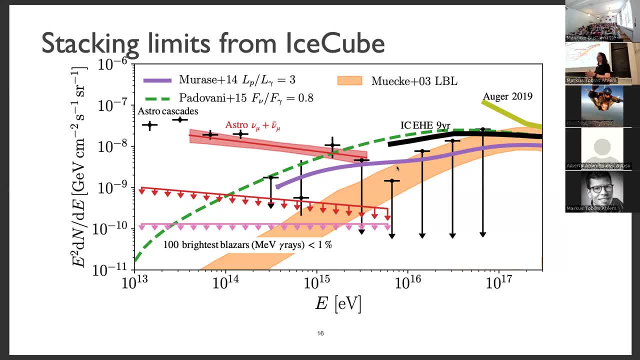 into the details of that. I can talk to whoever is interested afterwards. but anyway, So these are. they peak at lower gamma ray energies. This is somehow good for blazers to be more luminous And they found a very strong upper limit. 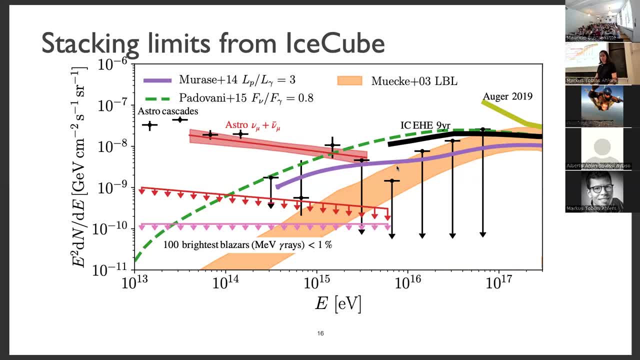 They found no signal. So there is now an upper limit of the order of 1% on blazers And then the lower limit of the order of 1% on neutrinosauruses, which is really constraining and a really you know. 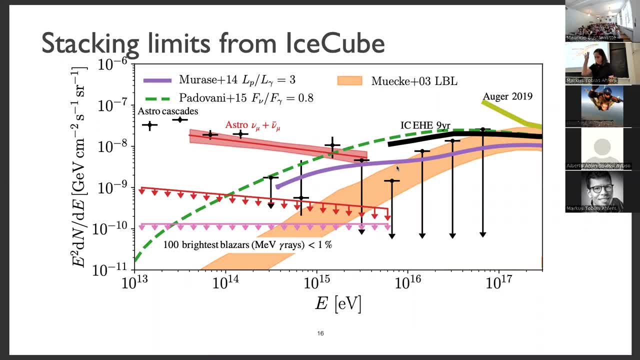 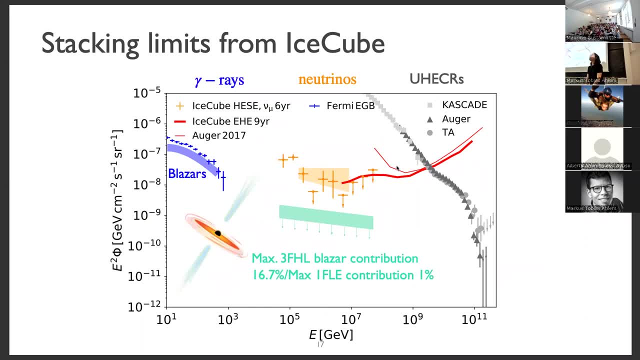 really important results which many people will be really struggling to interpret, including perhaps me. So, yeah, Yeah. so on the previous slides you have these model dependent predictions and you see the peak in high energy And then, when you're going to do your stacking, 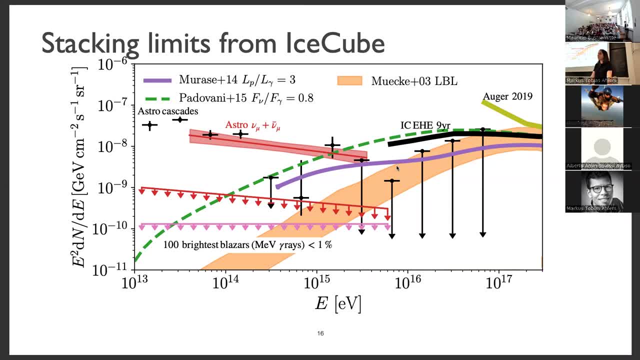 you see, it follows. so I see why they do it. but this puzzles me a bit that you have these models and then you're going to stack and you're going to show all the way, the data to be able to track the energy of the model. 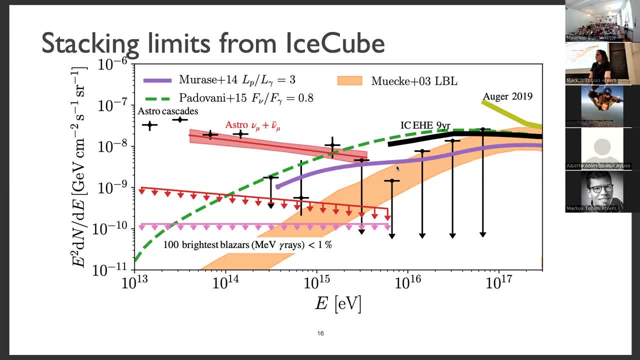 And then you have these models that you're gonna put on the plate, And then you're gonna put on the plate way the physics behind it. so I struggle how to interpret this upper limit. I was presented here when you know it should look different. 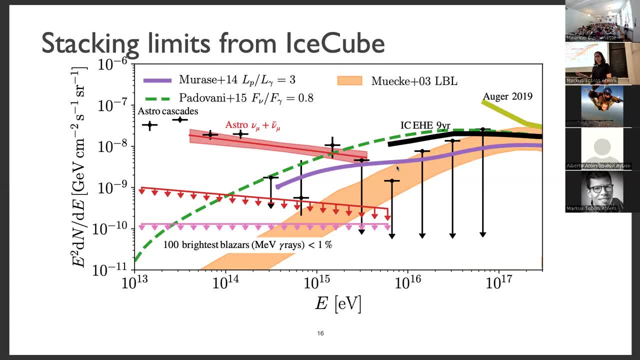 So this is, I think, a question for the experimenter. so I agree with you that. so for in this paper specifically, they didn't try Like, they only tried the need to the minus two, or neither the minus 2.4 or 2.7 power. 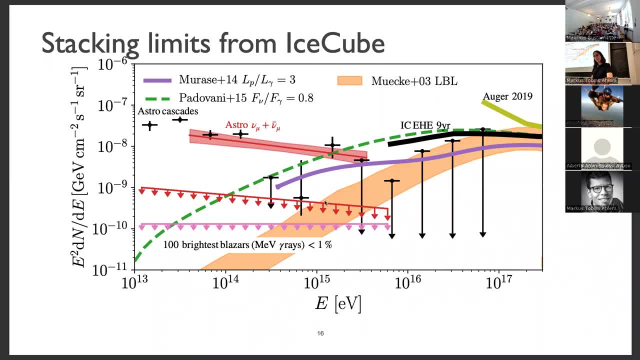 law. But I wonder what would the limit have been if they assume the need to the minus one power law? that would fit better, but I don't know if it would be that different, Marcus, to you. The high sensitivity is typically a 10 to the power, 14 electron volts. 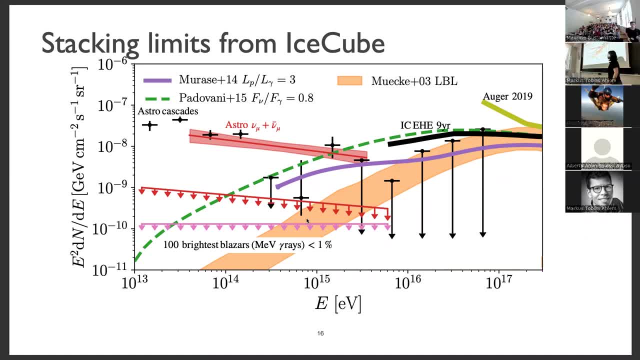 So if you have an e to the power minus two spectrum, it would probably then look like this here: Yeah, I mean coming close to this limit here. e to the power minus three would look like this: So you get like this, Yeah. 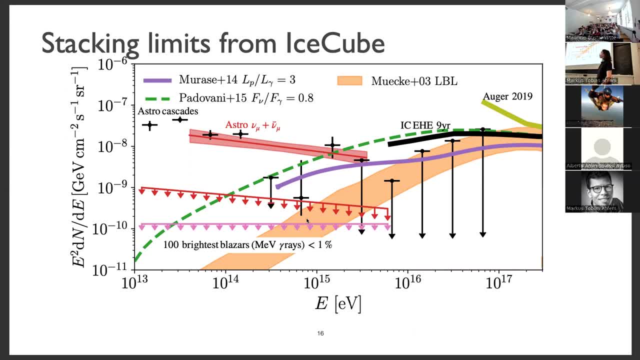 But of course you're right, If you have a good model for the mission would take the actual spectrum and fit it instead of having the power law and for example for gamma ray burst, we actually simulate the spectra and put in the combined limits after we wait this with the model specific mission, because 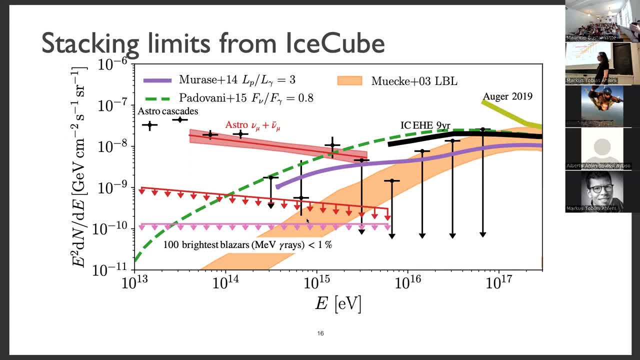 a lot of uncertainties and I guess this is one of the main motivation why many analogies are based on the simple power loss with two parameters: spectrum index and the normalization. And I just remembered that in this paper yesterday. they also show the differential limit and it has this U shape that Marcus described there. of course, the limit is not. 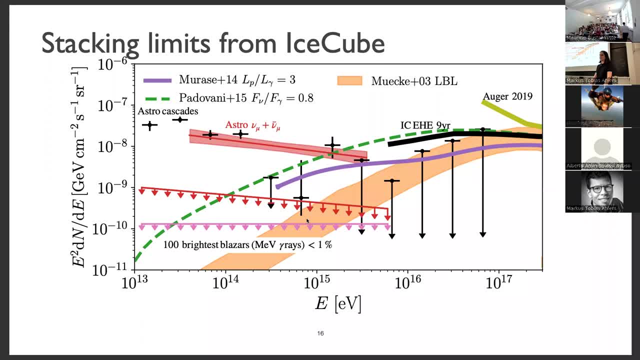 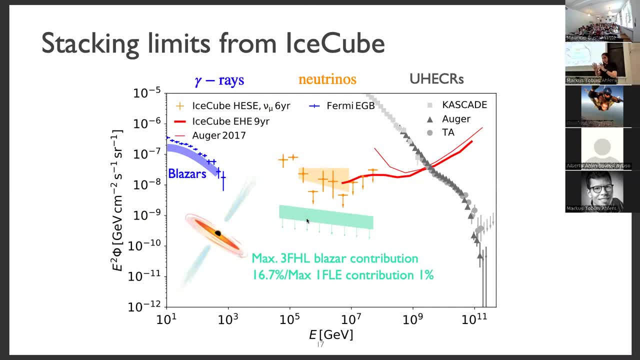 as strong as 1%, but still it's really constraining. So I don't know what it is 10%, but yeah, it's very constraining. and that's the main message. and I want to wrap this up by saying: remember that we started this discussion by 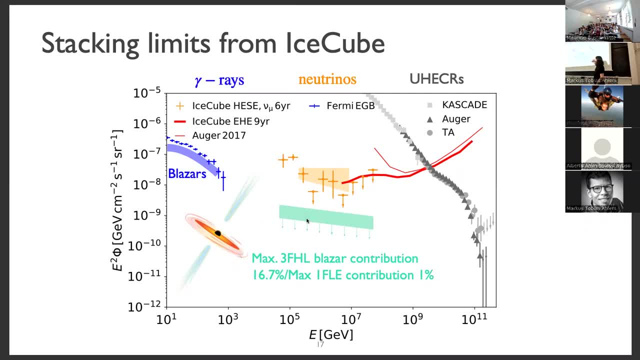 considering that the fact that all these different radiations, Diffuse radiations, Play sorry. gamma rays, neutrinos and cosmic rays, extra galactic ones, have a similar energy budget, We thought, well, maybe this is a sign that they all come from the same source: population. 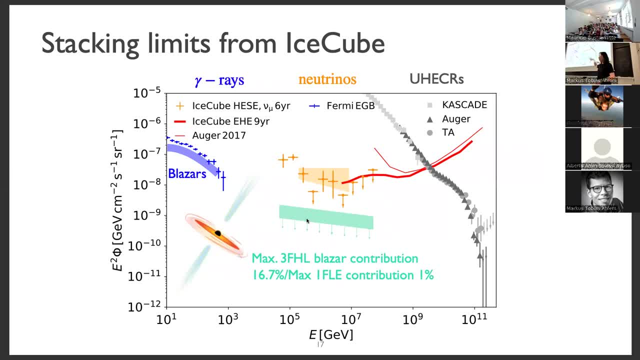 and we know that the gamma rays come from lasers, because we've seen there the major class of gamma rays, And we know that this is not what happens with the neutrinos. so we have really broken a very important Paradigm or possibility that many people liked, so that all the radiations do not come. 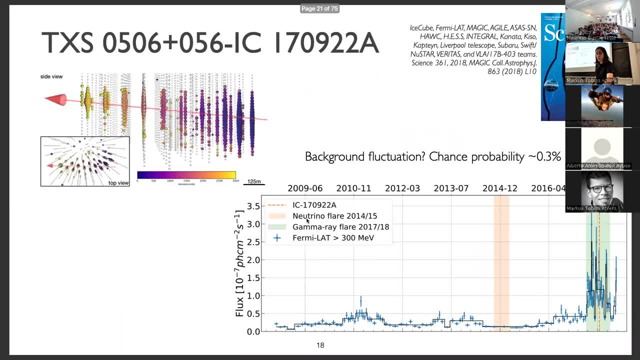 from the same source population. Okay, Now, this is not the end for blazers, and maybe most of you have heard about this. in 2017, there was a neutrino alert with the high energy neutrinos. when this happens, everybody gets an email- I get an email, you can sign up and get an email- and, importantly, those who have 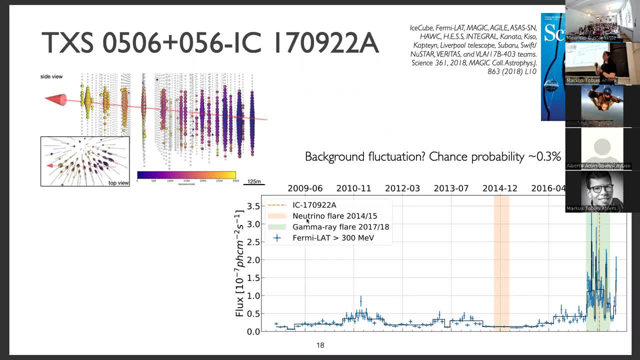 a telescope, They don't point. they point their telescope to see if something is happening in the direction of that neutrino. And in this case they didn't point because for me doesn't point, it just scans the sky. but what was quickly realized was that this is the gamma ray. 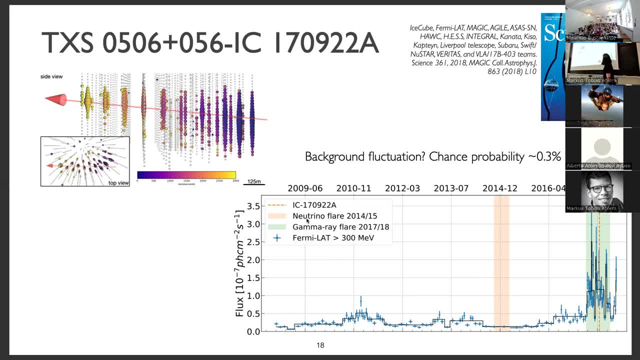 Oh yeah, here are the axes. so 10 years of gamma rays from this one laser. nothing was happening for 10 years. and then there was a six month flare, a really strong flare, and there was a neutrino Right there. that's the neutrino I'm talking about. 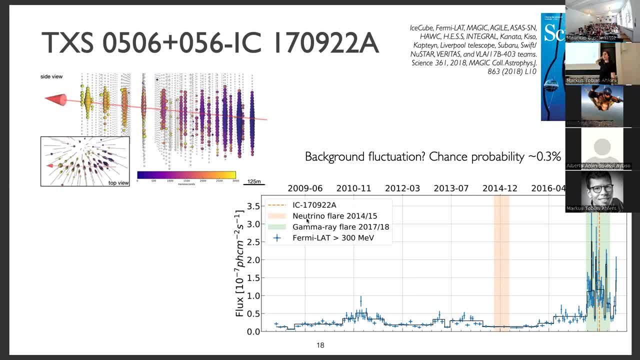 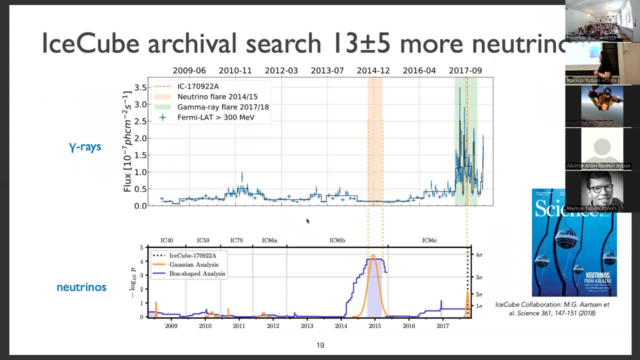 So the chance probability of such an observation is point 3%. So this was a very important moment for for our community and the first three Sigma access or point source: ice cube. So and later people will look back at the archival ice cube scientists look back at. 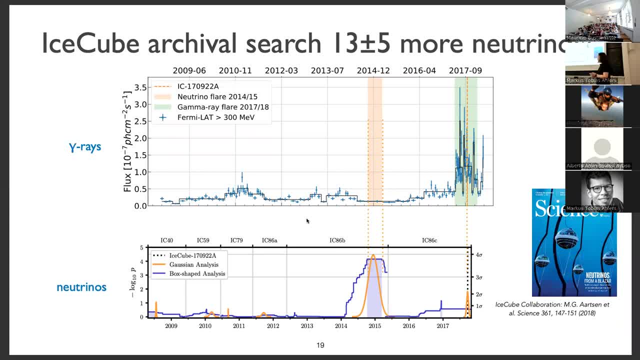 the archival data in the direction of that source And found that in 2015, 2014, there was a six month period during which there was a neutrino flare, So 30 of order, 13 neutrinos in excess of background, and that alone constitutes an independent 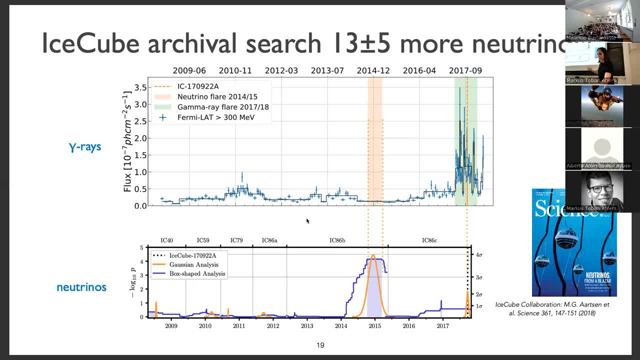 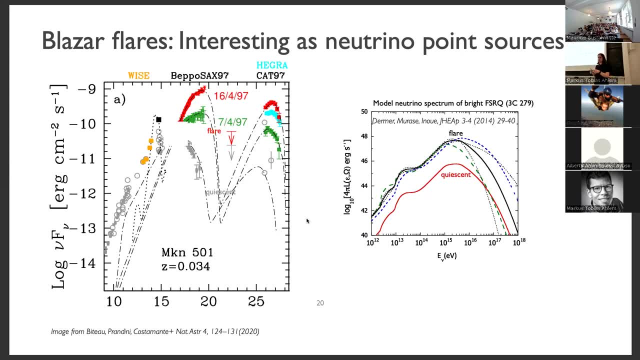 3.5 Sigma event. So how can we interpret this? so I just told you that lasers are not producing the bulk of the ice cube neutrinos. Now I want to tell you that, still during a flare, This is a flaring laser and during this flare it was gray before it flared. 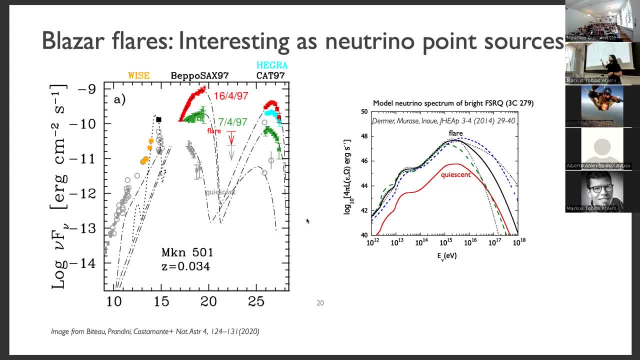 And during this flare it changed its flux by a factor of almost 100.. So, all of a sudden, even if this is not a very strong point source, it has a chance to really get bright. and during its flare- and since these photos may be the target for, 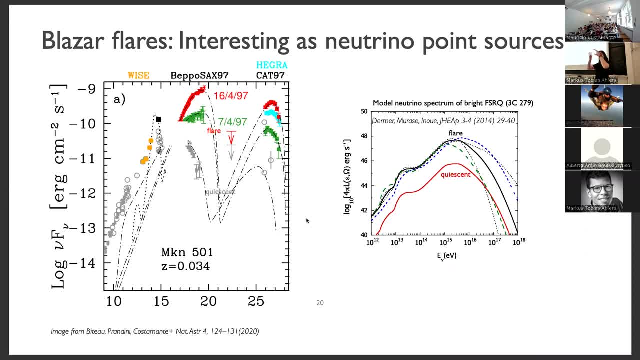 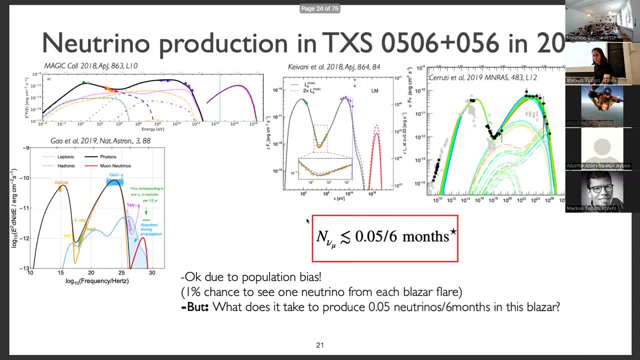 the neutrino. We have good reason to think that maybe the neutrinos are flaring at the same time, So theoretically this is very natural to expect. So this was a nice exercise that this community did. So. as soon as the alert neutrino was made public, all theorists were working independent. 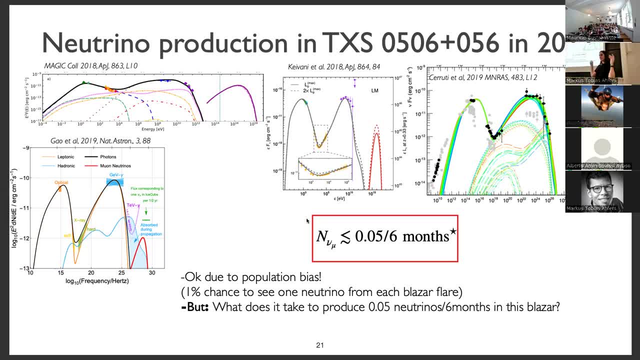 from each other and sort of in competition with each other, and they published their papers on the same day. And no, it's true, They published. They published the day after the ice cube publication, And what was very interesting is that everybody had the same results. 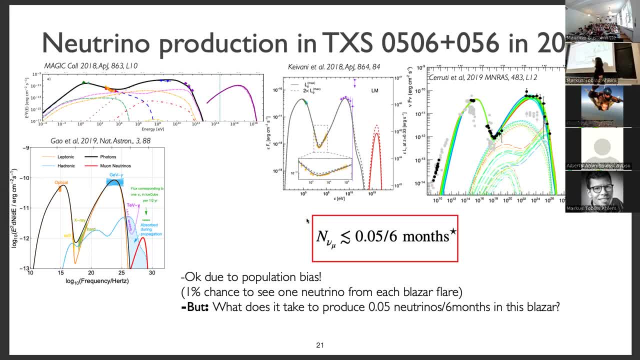 And what everybody found is that at most this flare can have produced a 20th of a neutrino in six months. So this is okay because you know the probability to detect this neutrino. to detect one neutrino, if I have, 0.05.. 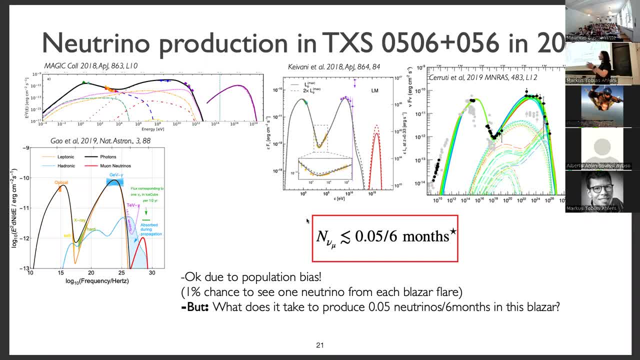 Expectation value is 5% of. if I have 20 such blazars, I expect to see one. However, what I want to talk about now is what it takes for this source to produce this flux of neutrinos and what limits us to that, to that number here. 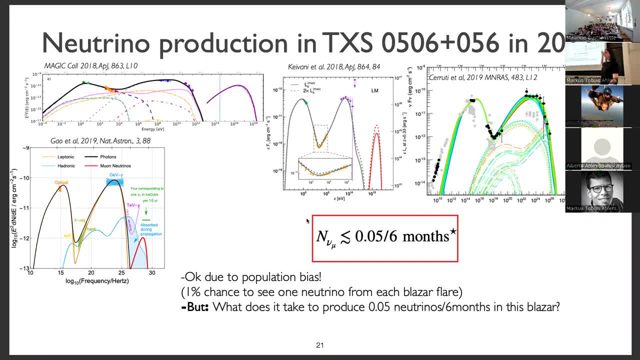 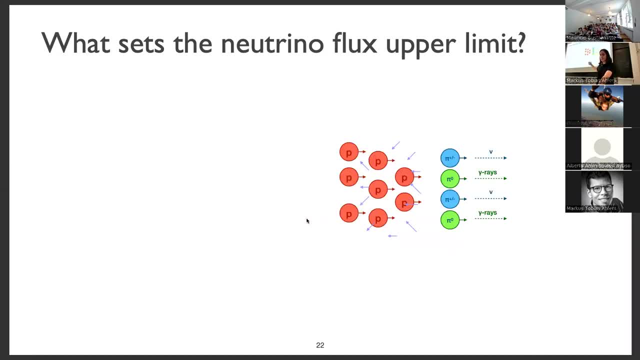 Why none of the of the groups working independently could get any more neutrinos out of this source. So here I want to remind you. So we're looking at photopion interactions. Of course, We have a lot of photons inside the source and these are, in a sense, one of the reasons. 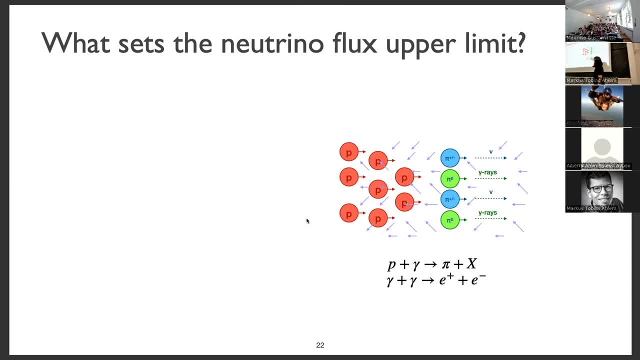 why we have an upper limit? because, since we have these photos interacting with our protons to produce neutrinos, these photons are also a target for the gamma rays from the neutral pion decay And these gamma rays interact quite a lot to produce electropositor pairs. 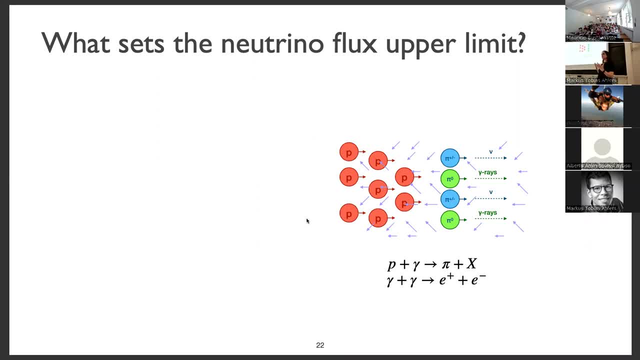 So the fact that this is a Strong gamma ray emitting source puts us, puts a limit to how efficient neutrino production can be in the source, because what is good for the neutrinos target photos is bad for the gamma rays. The gamma rays would be internally attenuated in this source, and so we can actually calculate. 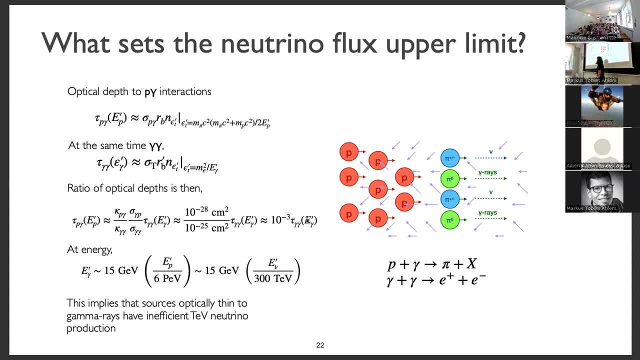 So we know the ratio of the cross-section times in elasticity of the two processes and we know that. So the neutrino Production efficiency Could not have been that high in this source. Now, if we had a 300 TV energy, this corresponds to a proton with six PV energy. 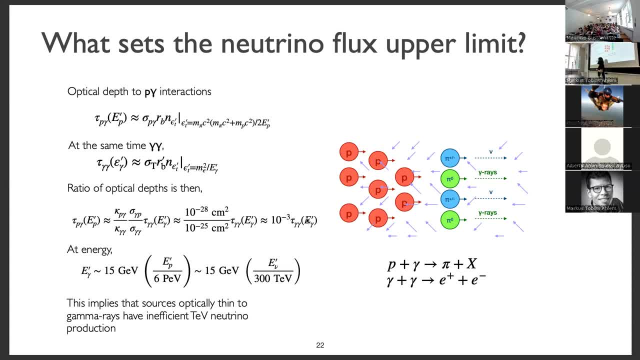 And we know that the target photons that this proton preferentially interacts with are the same ones as the 15 GV gamma rays. And the fact is, we saw a lot of 15 GV gamma rays. In other words, the neutrino production efficiency could not have been that high in this source. 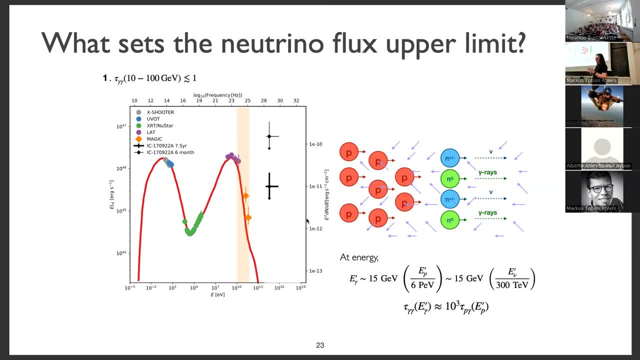 Now, if we want a lot of neutrinos, what else can we do If we cannot have very efficient neutrino production? Okay, We can buy brute force, increase the proton luminosity, This Sort of Tunable parameter that we can just put it up as much as possible. 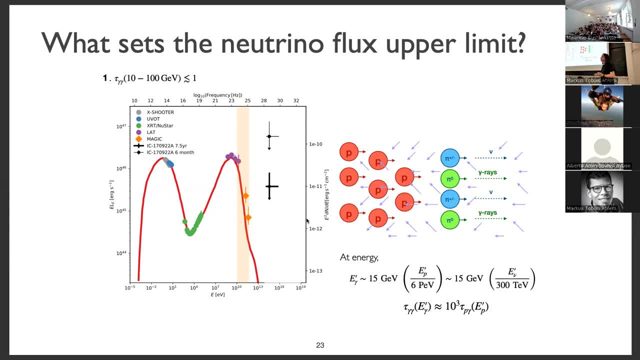 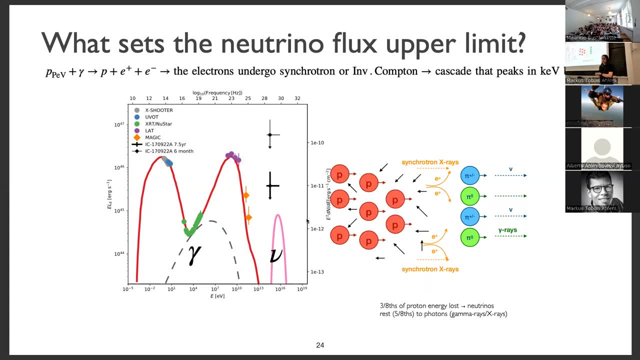 So if we can't make it deficient, we just inject more protons or assume that more protons were injected in this system. And this is another place where we get this upper limit to the neutrino flux. So while the proton luminosity increases, we increase the neutrino production, but at 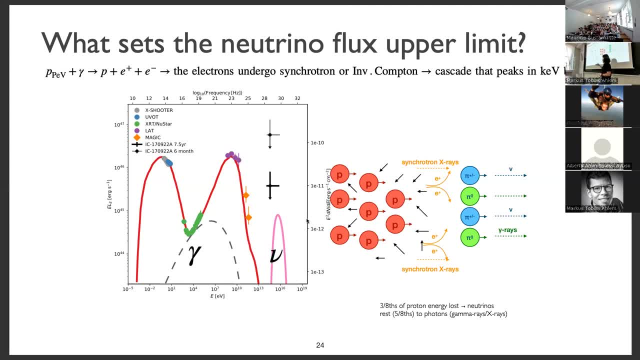 the same time we increase all the other, the photos that are produced in proton interactions. Right, So we have uh uh. we have uh electron positron pairs from the Heidler interactions. We have neutral pions producing gamma rays. 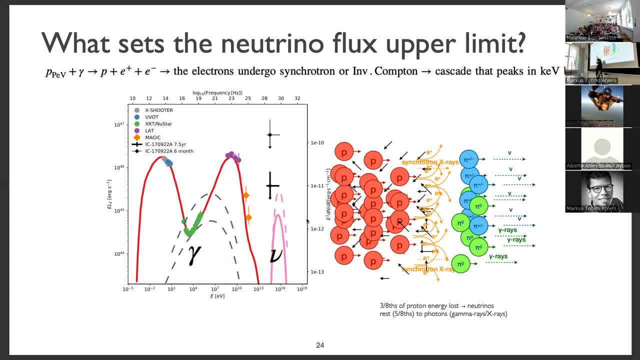 So at some point we're going to produce too many photons. Okay, So we overshoot the x-ray data, in this case, in this source. So this is what sets a strict upper limit to how many neutrinos this source could produce without violation. 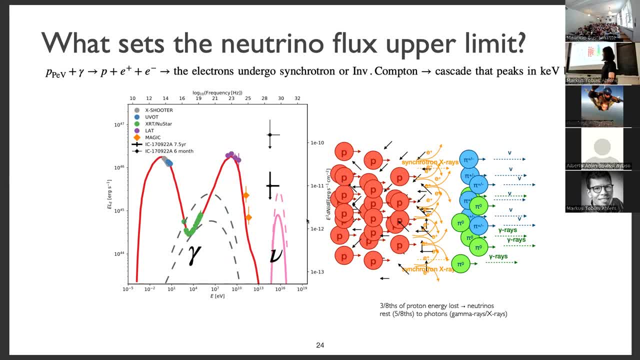 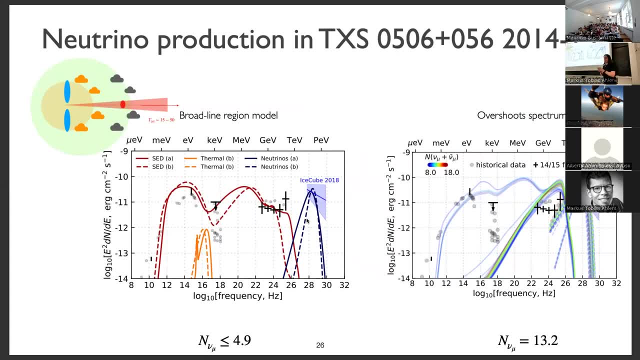 Okay, So this is what sets a strict upper limit to how many neutrinos this source could produce without violating all the constraints we have from x-rays and gamma rays. Okay, Okay. So, all in all, my conclusion here: if this source produced this neutrino, it's a statistical 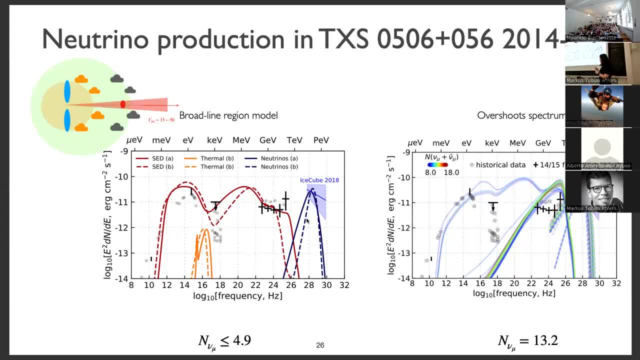 fluctuation that we observe it. Another thing that I didn't say but I can say now is that the proton requirements are extremely high and cannot be representative of the entire blazer population. So maybe this is a kind of rare event In blazers but it cannot be what happens in all blazers or we would have seen a lot. 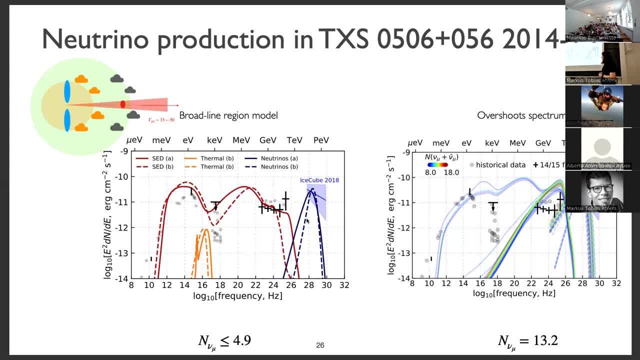 more neutrinos from the whole population. Um, now the 2014 flare- remember these 13 neutrinos- is even more of a mystery. So several groups tried to model this one as well. And if they, again, by brute force, increase the proton luminosity enough so as to get 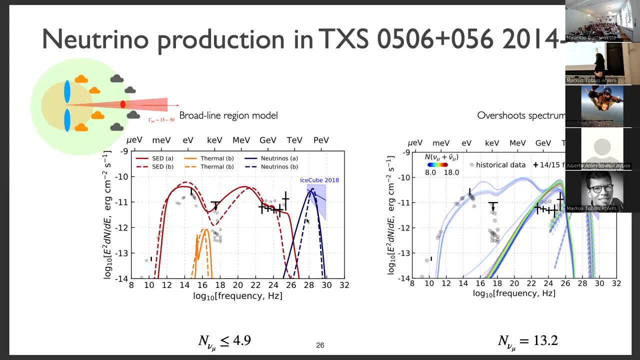 13 neutrinos, as is shown here. They violate the gamma rays. They violate the gamma rays and the x-rays. So so far there isn't. there are things that one can invoke and say there are more photon fields and so on. 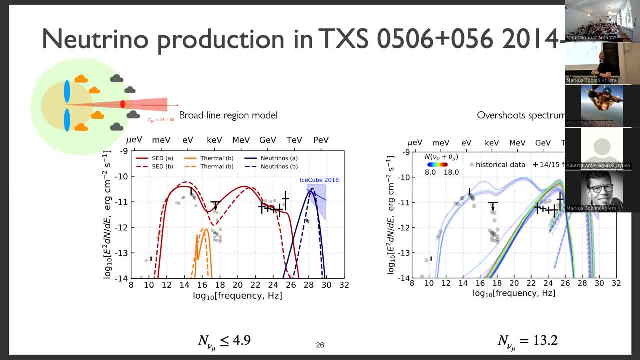 And um, but it's really very um, extreme parameters, Yes, Okay, Good one, Uh, but how do we show that neutrinos and gamma producing neutrinos? Uh, I think that's a good question, Okay, So how do we show that neutrinos and gamma produce in the same zone? 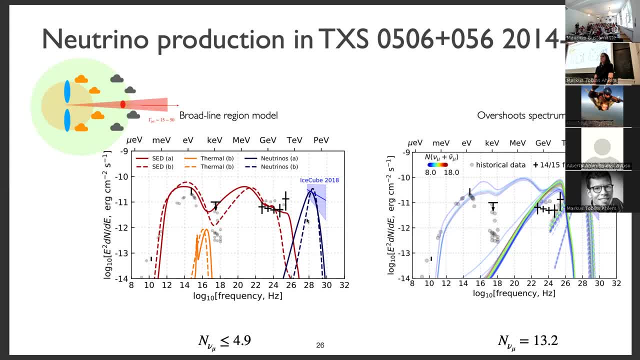 At the same place. no, if we relax the requirement of having a single zone, Well, first of all, wherever I mean where neutrinos are produced, some gamma rays have to be produced, and then we can start to add parameters to our model and eventually increase neutral production. 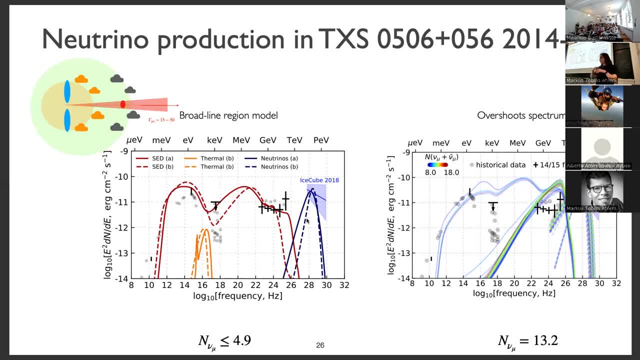 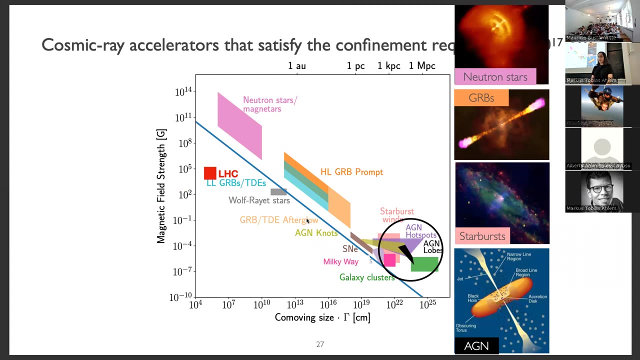 a little bit with respect to what I showed here, But the general picture is that we need proton content, which is extremely high and and typical of the laser population, So this doesn't change. Okay, this is what I wanted to say about lasers. 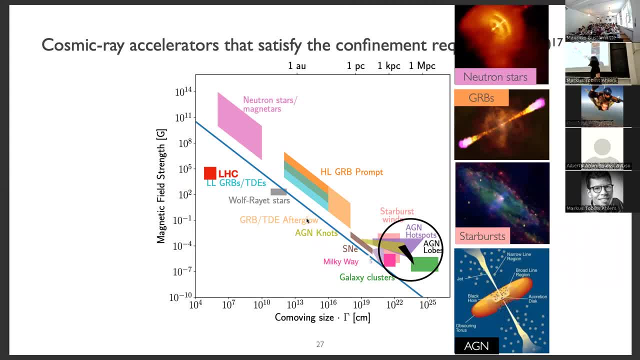 And now I want to briefly say So. you see that all these here- I call it Aegean lobes and hotspots and so on, All these are regions in the in the in jetted Aegean. The lobes are the outer part of these jets and these are all places where we can comfortably have production of very high energy cosmic rays. 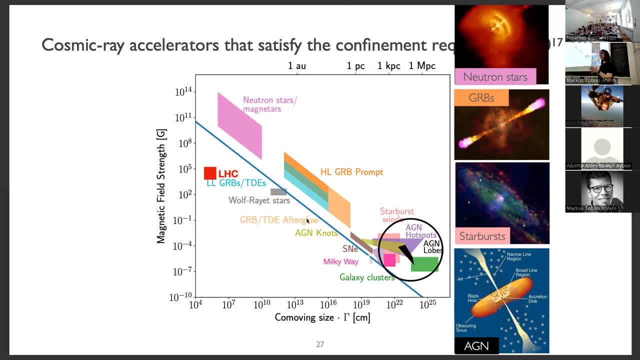 But I want to briefly say another thing about Aegean. Remember that on on Monday I said that only 10% of Aegean Had jets and only a small fraction of those jets are pointing towards us. So people already in the nineties said, Well, why don't we consider the neutrino production in non-jetted Aegean? 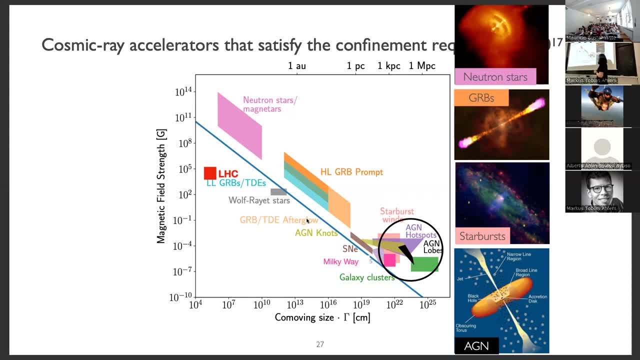 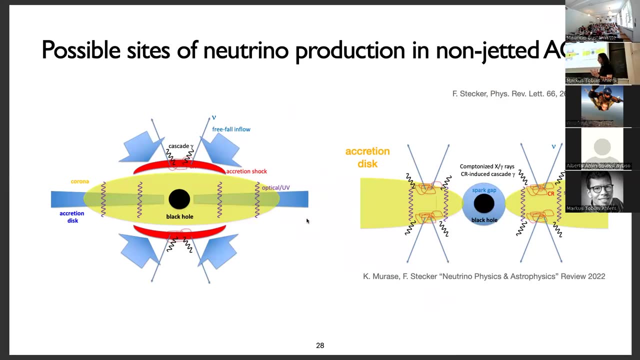 So they don't have a jet, So it's not so clear where they produce the, the protons, but they are more numerous, So maybe their total contribution is important. So here the models are. I would say, not a standard, No, but then the the most sort of accepted scenario is that, as we have been falling matter into the supermassive black hole in these jetted Aegean and there is pressure coming from all the radiation and particles close to the black hole, 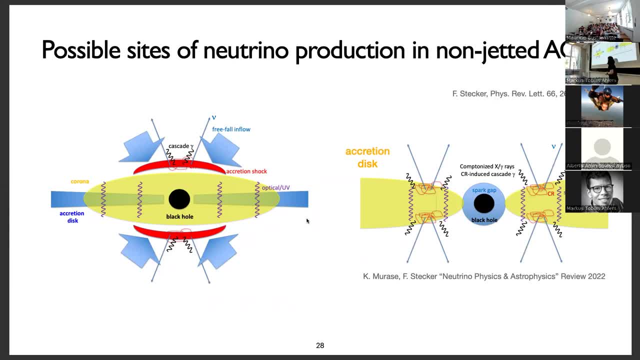 we end up with a shock surrounding the accretion disk. So people in the nineties already remarked that there must be neutrinos. So we have this standing shock. This is where we accelerate cosmic rays, And then we have all these photon fields related to the accretion disk. 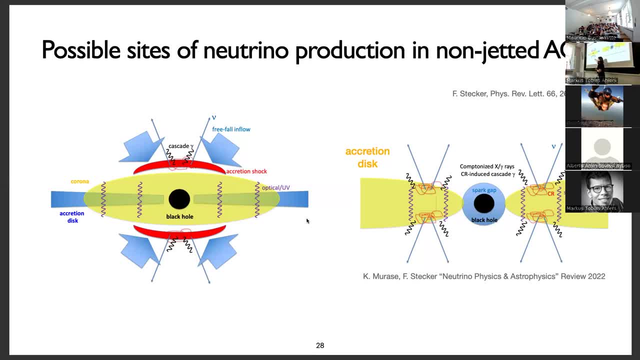 This is where neutrinos can also be produced. So in the course of Aegean and when this happens, we have so many more non-jetted Aegean than jetted Aegean that we expect the strong neutrino signal. 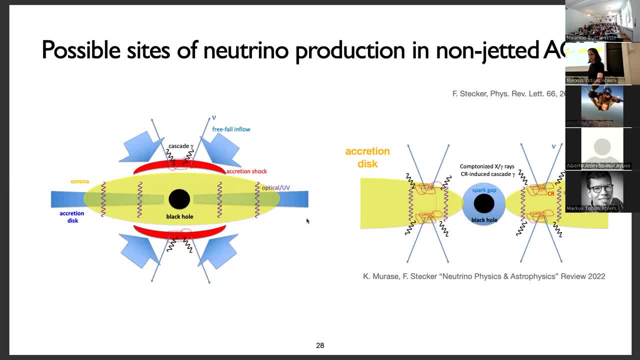 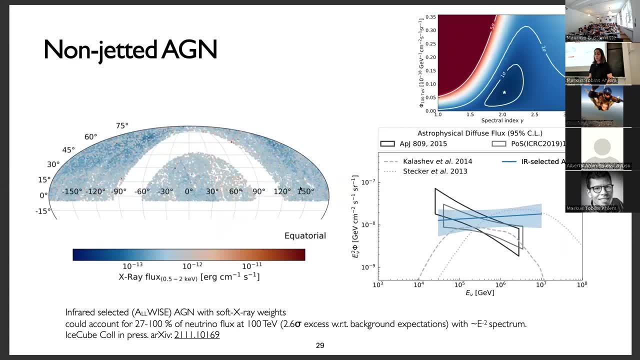 So that that was the paper in 1991.. And so recently there has been one, What I think is a very interesting result from IceCube. So they stacked the positions of all non-jetted Aegean from some galaxies And they found a two point sigma excess with respect to background expectations. 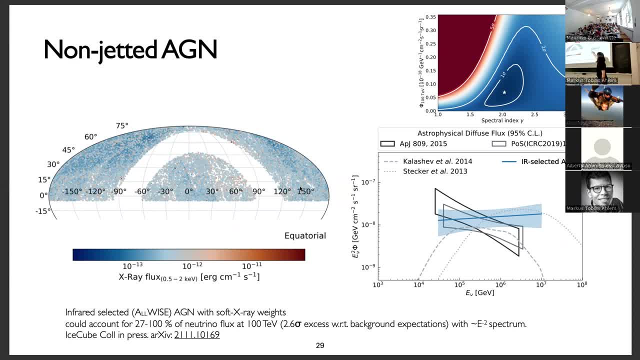 And what I find really nice is that the spectral shape that they infer is this blue shape here And it's almost e to the minus two parallel. So also what you would expect from astrophysics: the shock acceleration you see here. this is the model. 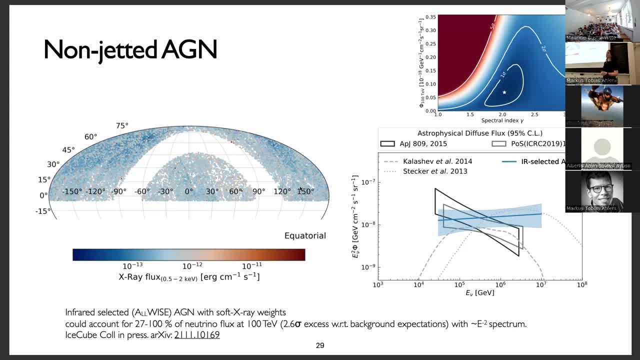 So actually this is really nicely on top of that model. So I find this compelling, but it's only two point six sigma And maybe someone from IceCube here can tell us this will take a long time, I think, to grow. 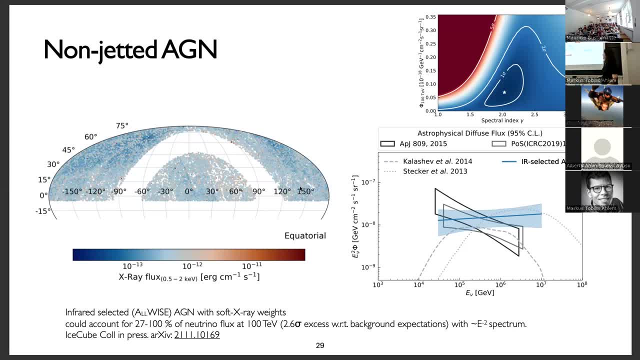 I'll be certainly looking out for what happens with this. I don't know, Marcus. can you tell us? will it take many years? So this is a recent analysis, So I guess you would have to double the data to get above three sigma. 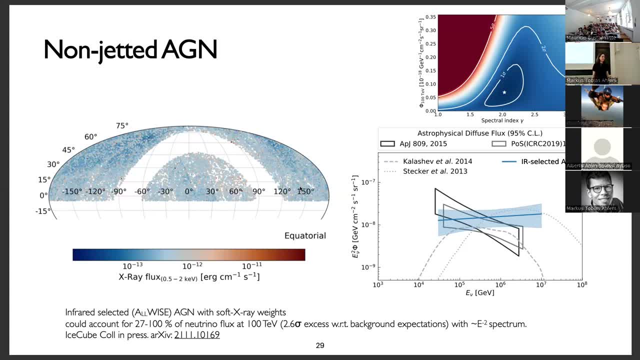 Yeah, And of course, two point six sigma. I mean this is high chance. I mean I don't want to down talk. Yeah, I understand It's interesting, But yeah, it's still. the verdict is out. We need to wait at least, as you said, double the time. 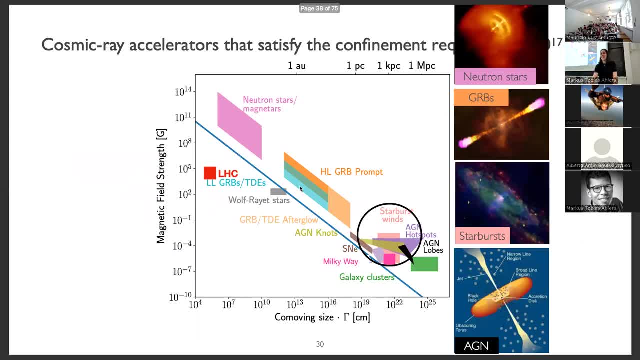 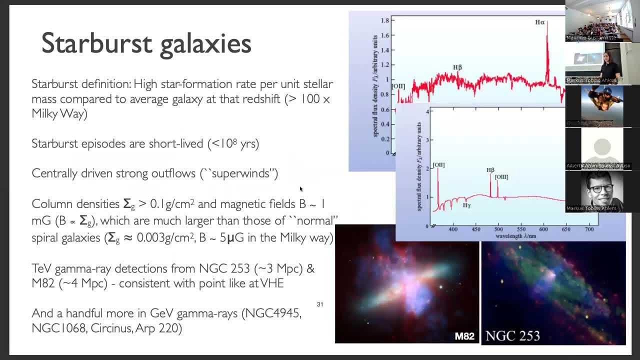 So, yeah, OK. so then I will not talk much about starburst galaxies, because Enrico will talk about them. I had prepared just a couple of slides, just the main, OK Thing to remind you here is that we see these really crazy emission lines which tell us that there is a lot of gas, a lot of star formation. 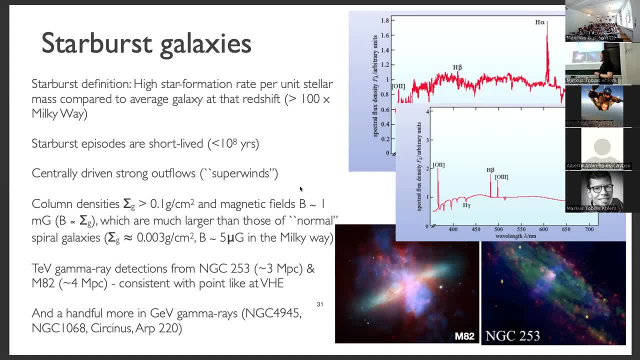 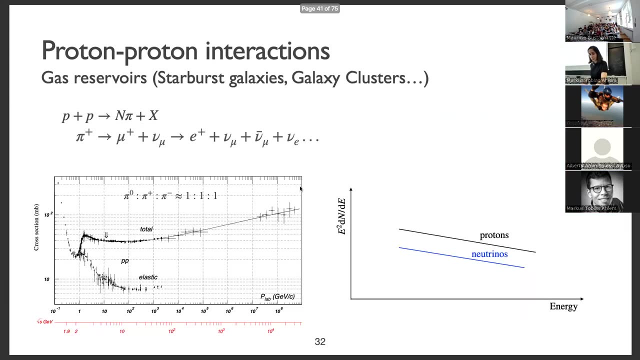 There's also cold gas. This is what enables star formation, And this is great, then, for for the production of neutrinos The magnetic fields are strong. This means cosmic rays are trapped in these galaxies for a long time, And some of the nearby starbursts have been seen as gamma ray sources. 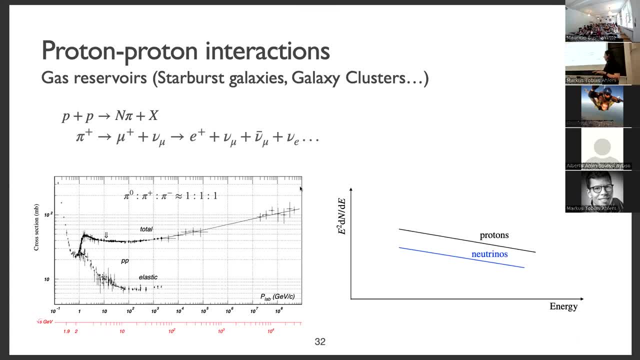 One thing I want to to remark here is that, unlike photopion interactions, where we get this very peak spectrum in starburst galaxies because they have all these, these thermal protons, the most likely channel for neutrino production is then proton, proton interactions. So here the cross section is flat, as you see. 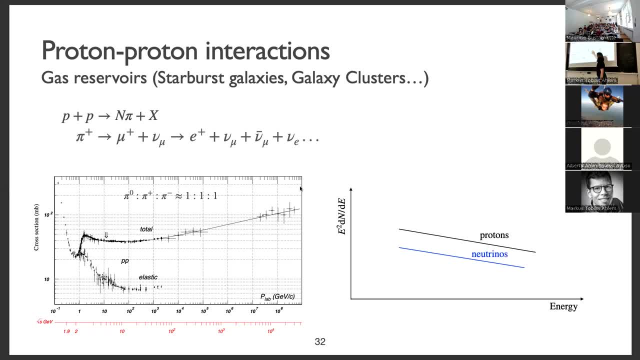 And so, as a result, if we have a power law proton spectrum, then We expect a power law neutrino spectrum, And you, you know, this is not so different from what ice cube sees. So in that sense this works. 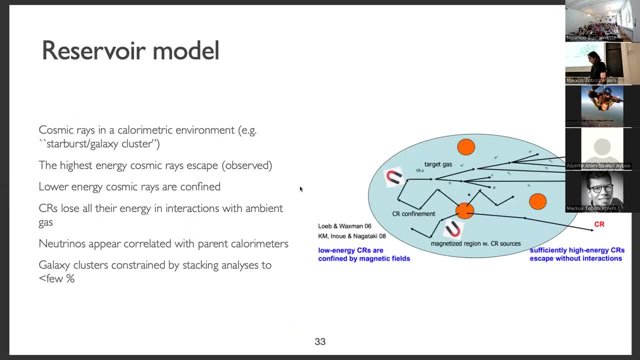 And so I just want to briefly say that starburst galaxies- but not just starburst galaxies, also Euler's and also galaxy clusters, have been proposed as good environments for having what is called the reservoir, The reservoir model in which we have acceleration of very high energy cosmic rays. the highest energy cosmic rays have the largest llama radius and they escape their sources. 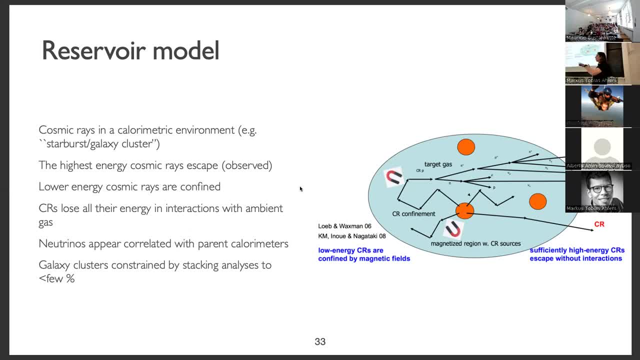 The low energy ones are trapped in the magnetic field of the source and they stay there and they interact a lot and they produce neutrinos. So in that sense we we could have A situation in which a single Population under the reservoir model produces both the ultra high energy cosmic rays and a very strong flux of neutrinos. 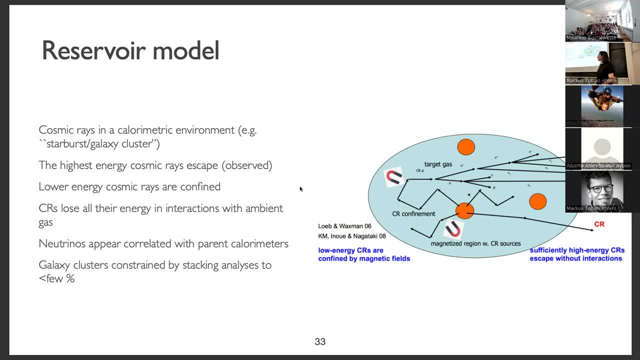 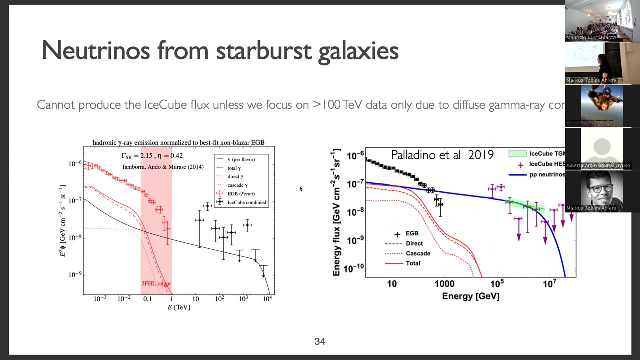 And I think this is still consistent with more or less everything we know about the neutrino. So this is not ruled out, that this happens in some of these sources. And just briefly to say the only problem with starburst galaxies is that If we want to explain all the neutrino data, with starburst galaxies down to low energies- 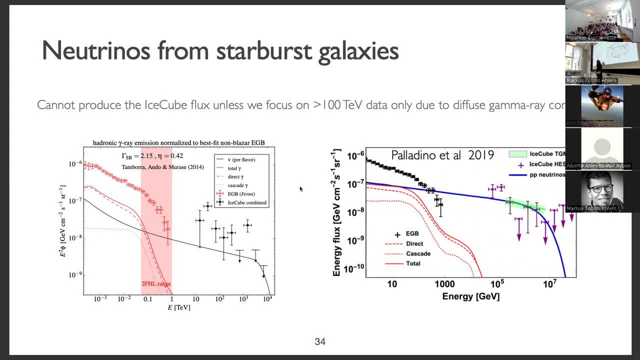 We have a problem, and this is that they would overshoot their the diffuse gamma ray emission that they are allowed to contribute to the total diffuse gamma ray emission that we see after we've subtracted the blazers. So this is a problem for starburst models, but the fun is happy to give up on these low energy. 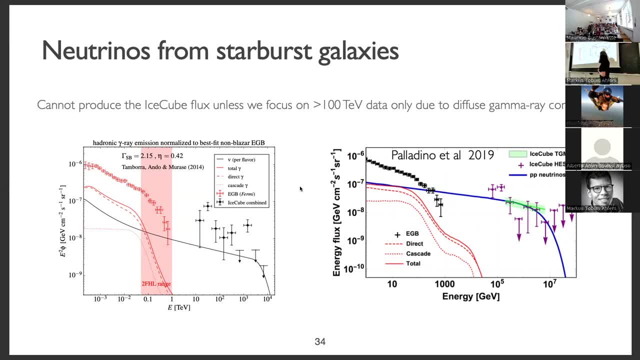 So this is a problem for starburst models, but the fun is happy to give up on these low energy data So and say that they come from some other population. then the medium energy data- or I don't know, this is not the correct term- the high energy data in ice could be- are consistent with starburst galaxies. 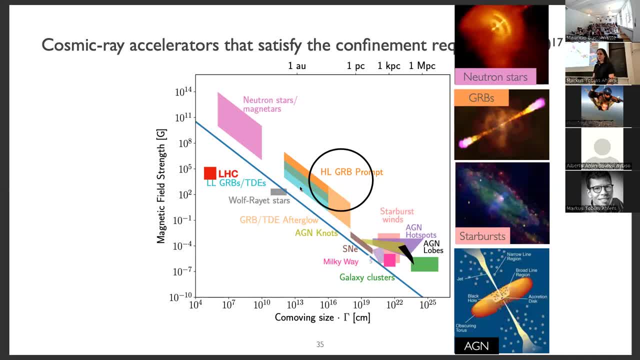 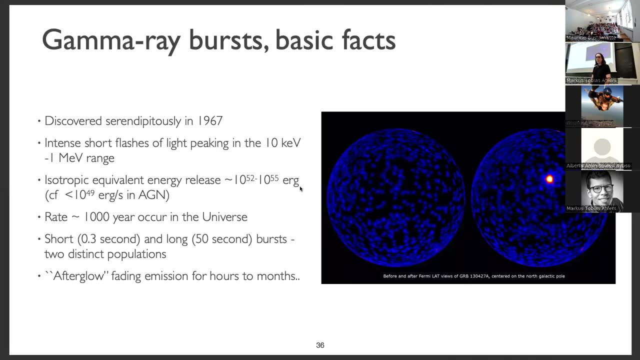 Okay, so now I will switch to gamma ray bursts. these are another one of these populations that everybody thinks must be doing some high energy, cosmic ray production, because they have these extremely collimated jets. So for those, So for those who are not so familiar, so these are very strong pulses or explosions which 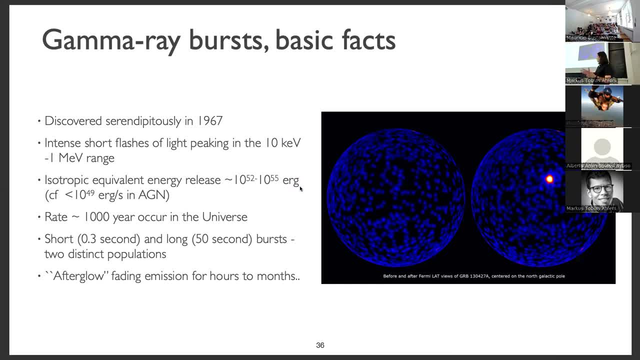 last a very short time. They last from few seconds. Actually, we see a bimodal distribution. Some of them last half, or not half of them, but one population lasts less than a second and we call these short GRPs. and then the long ones last almost a minute. 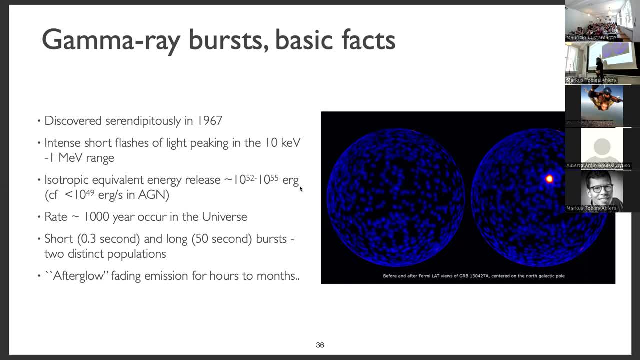 And during this time they release energy up to 10 to the 15 ergs. So compare that to the brightest AGN, which is 10 to the 49 ergs per second. So for a brief time, they are the most powerful things in the sky, the most powerful gamma. 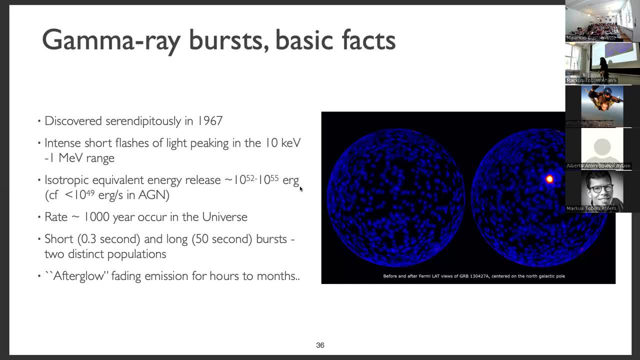 ray sources in the sky So truly remarkable. And in addition to this prompt phase, of which last is less than a minute, they have fading emission which goes on for months, And now there have been three of these gamma ray bursts that have also been seen as TV. 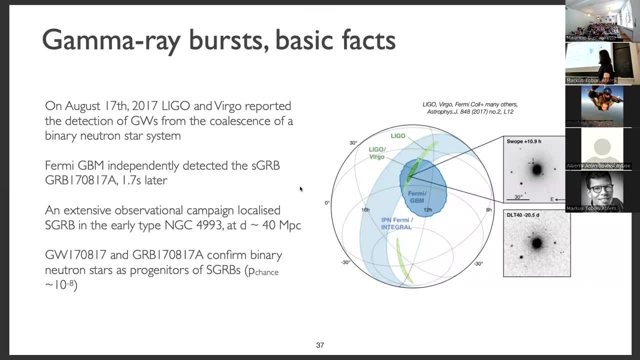 gamma ray sources, And so perhaps the most important result associated with these GRPs is that in 2017, when LIGO reported its first detection of these GRPs- And this is the first time we've seen this- This is the first time we've seen a Newton star merger event. 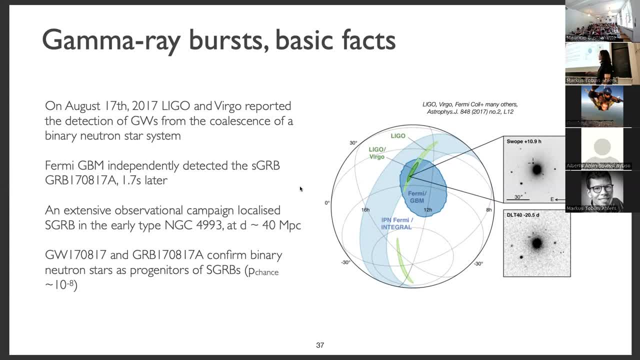 Within two seconds, the instrument in Fermi which looks for GRPs found a GRP And, after an extensive campaign with optical telescopes pointing to look for the host galaxy, they found a host galaxy which is about 40 megaparsecs from the Earth. 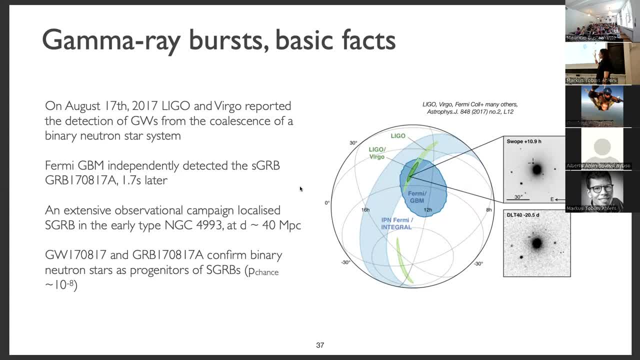 The host galaxy in which we now think both the neutron star merger and the short GRB originate. So this was very important, because for many years people thought that short GRBs are the product of neutron star mergers, but nobody had any proof. 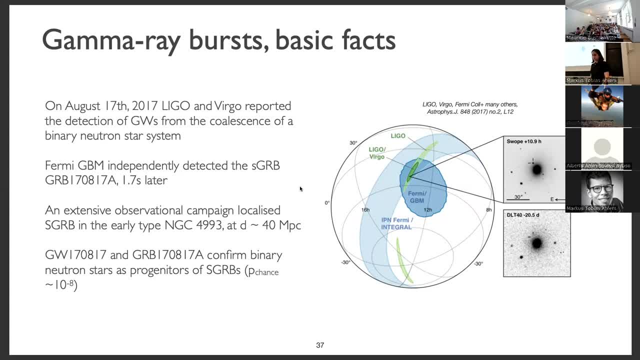 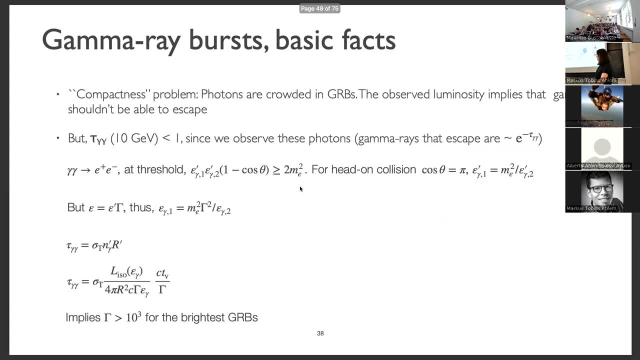 So this was proof of a very well-accepted model and a very important moment for multi-messenger astronomy. And one thing I want to say here about GRBs is similar to what I was saying before about lasers: The fact that GRBs even exist tells us something. 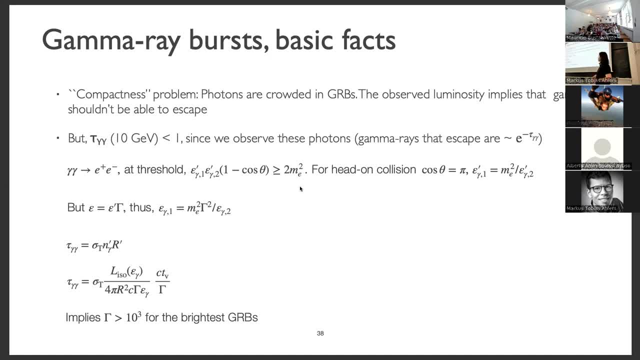 about how relativistic they are. So we measure 10 GV or higher photons from GRBs, but we also measure their size from the fact that they are from the timing, So we can figure out how much the shock can or how much this matter from the explosion can travel. 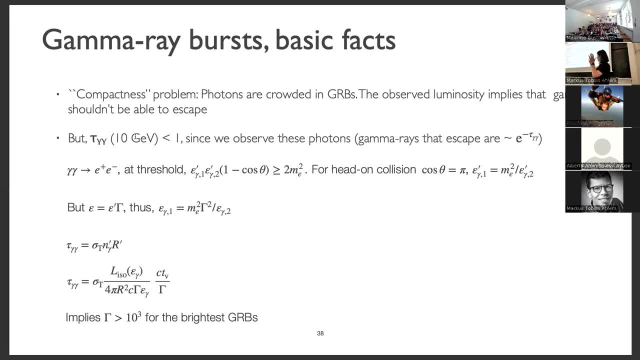 in a certain amount of time. that gives us the size And we measure luminosity. This is our observation. So putting together these two, we can work out the number, density of photons in that region where the GRB happens, And that is so high that the gamma rays should not be able to. 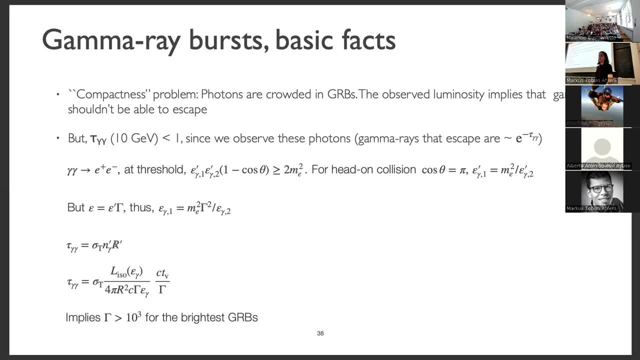 and that is so high that the gamma rays should not be able to, and that is so high that the gamma rays should not be able to to escape. And the only thing which we can change here, when we calculate the optical depth, which is radius, 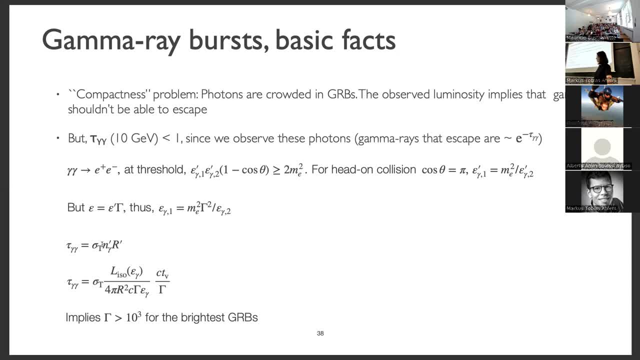 So the size of the region times the number density of the photon targets times the cross section is how we- whether this is a very relativistic source or not. In that case our inferred number density is larger than the density in the rest frame of that source. 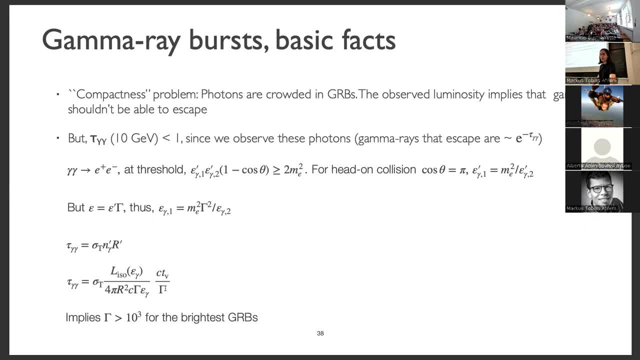 And so from that you see here that the factor of gamma squared appears, And so if that gamma is really large, then we can reconcile our observations with the fact that the gamma ray- yeah, So we can sort of live with the fact that gamma rays escape. 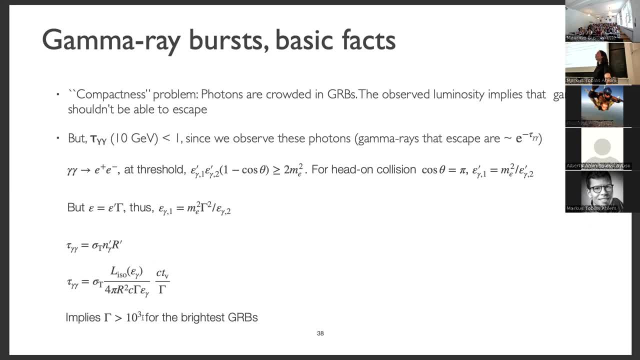 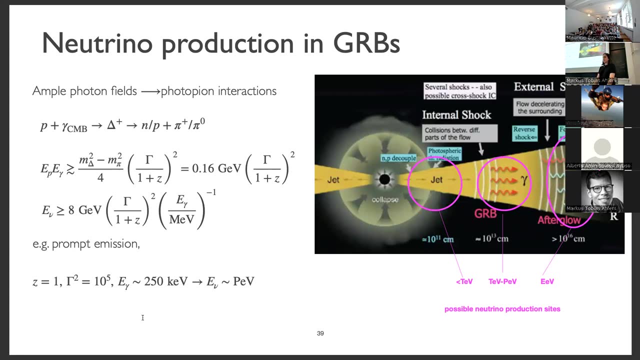 And this tells us that the Lorentz factor is of order a thousand for the, so extremely relativistic, much more relativistic than any Jette De Gea, for at least a short time. And so, as a result, there are many possibilities. 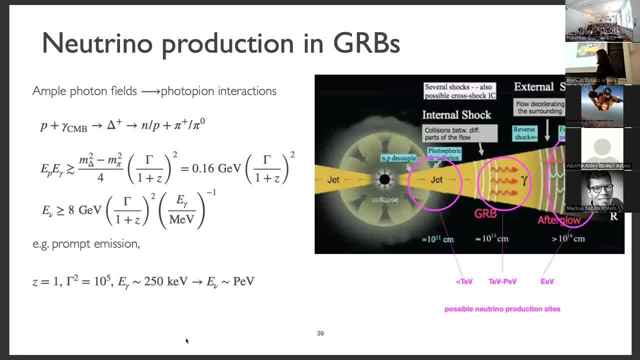 for acceleration of protons in this relativistic Jette. And so again, as I was saying before, depending on which time and which place in the Jette the neutrino production happens, We also have a different expected peak neutrino flux, because initially the photons are high energy. 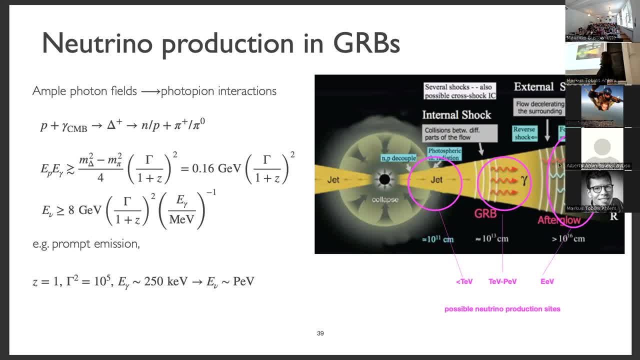 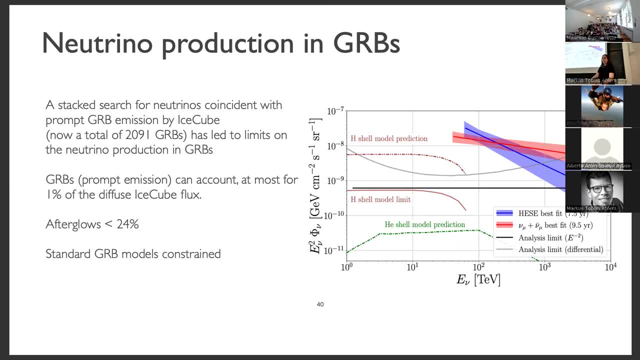 and later, further out, we get lower energy photons And so we expect, as a result, higher energy neutrinos. So here again, IceCube. this is a very important result from IceCube. IceCube has put very strong limits on GRBs as sources of high energy neutrinos. 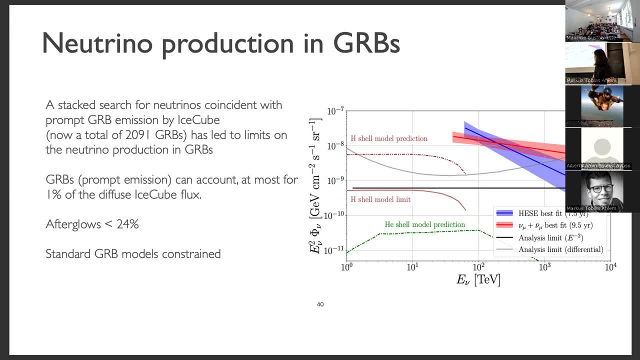 which was again a very surprising result. So with the stacking analysis that I explained before, IceCube is able to constrain anything more than 1% of the total neutrino flux coming from the prompt phase. So the first one minute of the GRBs. 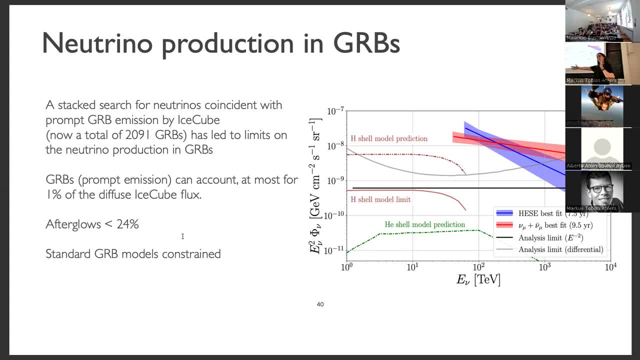 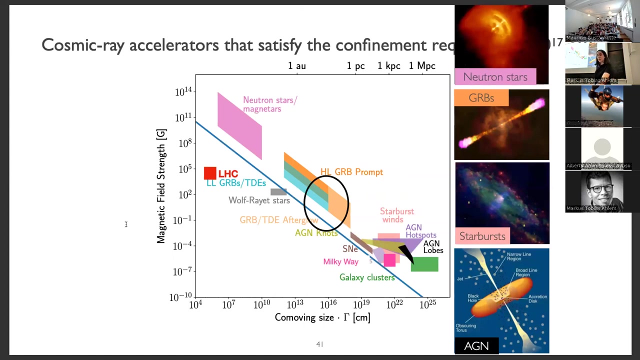 and the limit gets weaker as we increase the time window of the search. So it can be at most further 20% if we also consider a week or so the afterglow. Okay, so another very popular source, very strongly constrained. 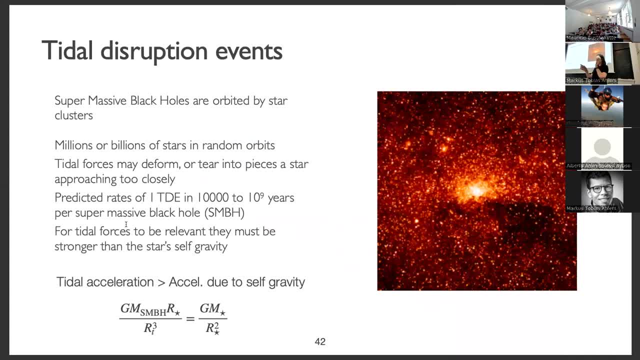 Related to these are tidal disruption events. So these are events in which, near the center of any galaxy, we have a huge amount of stars, and maybe you have seen around Sagittarius A-star- it's beautiful- orbits the 70s that roughly once in every 10 to the 4 to 10 to the 9 years, one star will be in. 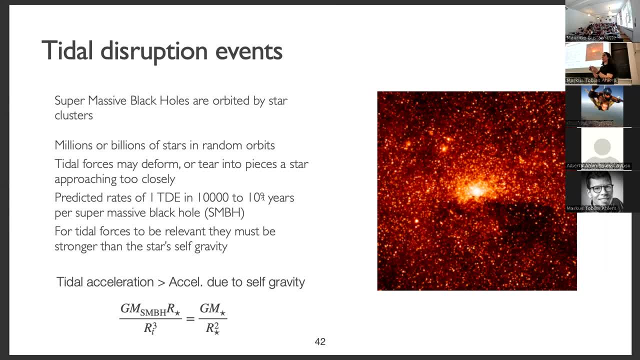 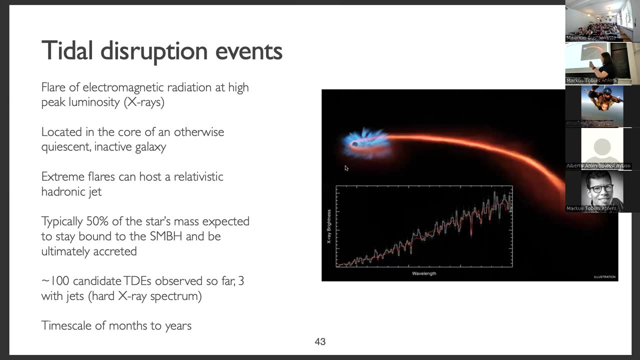 a situation where the tidal forces on it are larger than its own self-gravity, And so in that case the star is stretched and we have something like this, So we have a stream of star matter being pulled and then half of the star sort of ends up. 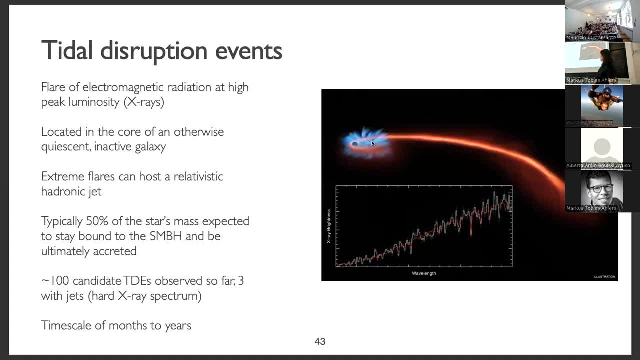 orbiting the supermassive black hole in close orbit and the rest in this sort of more open orbit, And this produces an incredible explosion. Now, this should happen in all galaxies, But if it happens in an AGN, remember, this is a very variable. 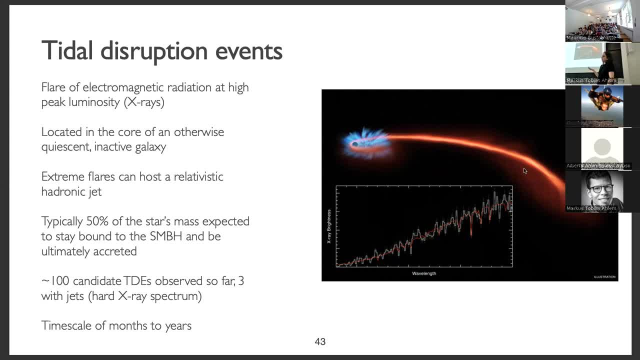 Galaxy, then we won't be able to detect it because there is intrinsic variability. So the best place to look for these is quiet galaxies where not much is happening. And so far this is a relatively newly discovered class of explosions. Observationally we have seen about 100 so far and now three of these hot jets. 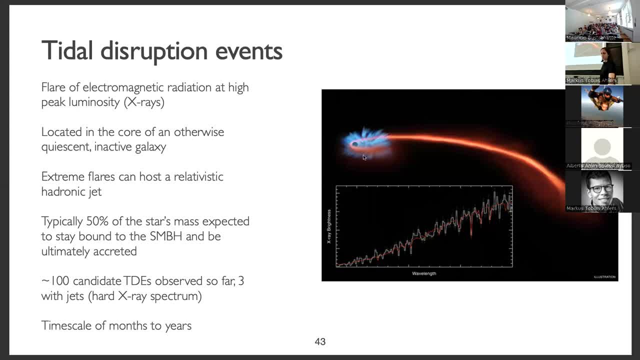 So what does this mean? So, OK, I showed here that what we end up with is this stellar Matter ends up forming a kind of accretion disk around the black hole, And in some instances we can have a jet in the in the polar direction, something like a small 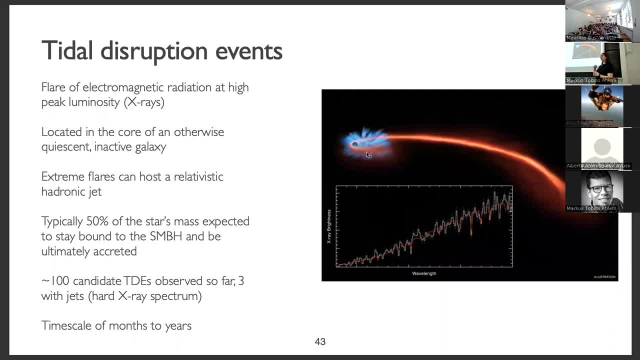 AGN jet basically, And if we have that, then it's easy to imagine that there's particle acceleration in that jet, And so, as a result, at least jet tidal disruption events have also been proposed as very good sources of high energy neutrinos. 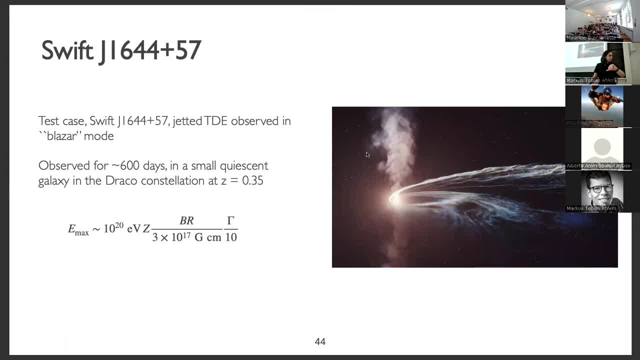 And, Okay, I have about 15 minutes, okay, Okay, but maybe I can go a bit faster, But so so, specifically one event to this in 2016,, Swift saw one tidal disruption event which is kind of the most beautiful tidal disruption event we have seen in Blazor mode. 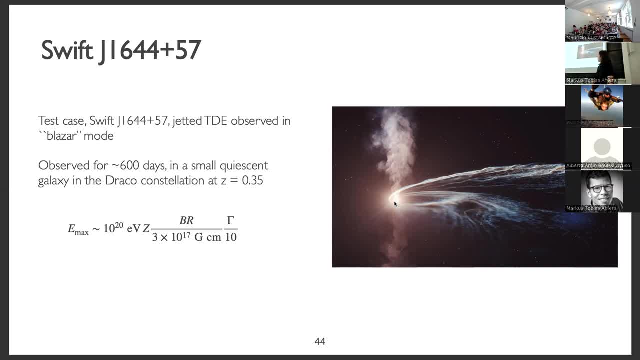 So we were looking into the jet And so for that event There were no neutrinos neutrinos associated with it, But the modeling that was done, which constrained the magnetic field strength and the radius of the size of the region in the jet sort. 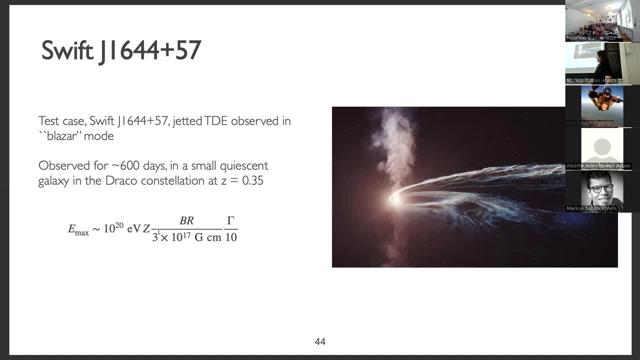 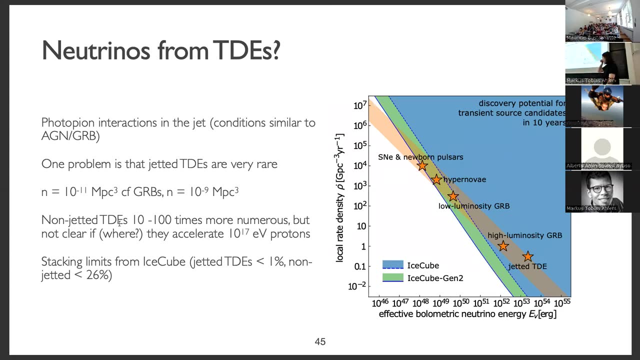 of? was allowed people to say that maybe even ultra high energy cosmic rays can be accelerated, based on the simple Hillis argument that we've used throughout these lectures? Okay, Now what do we know about neutrinos from tidal disruption events? So the process is similar to what I was. 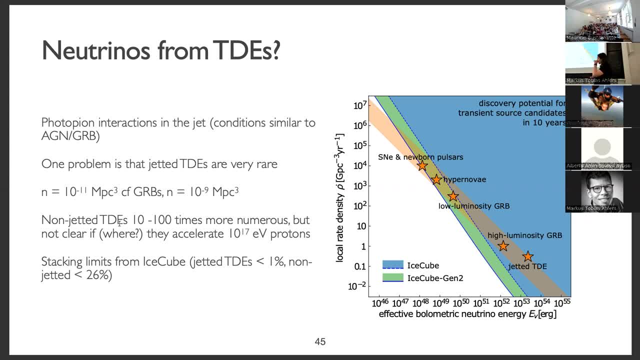 explaining before for blazers, for the pine interactions in the jet. But you remember this plot that we looked at and which Catherine also showed us, in which, since we haven't detected any point sources, we can rule out extremely bright and rare source classes as producing the ice cube neutrinos. 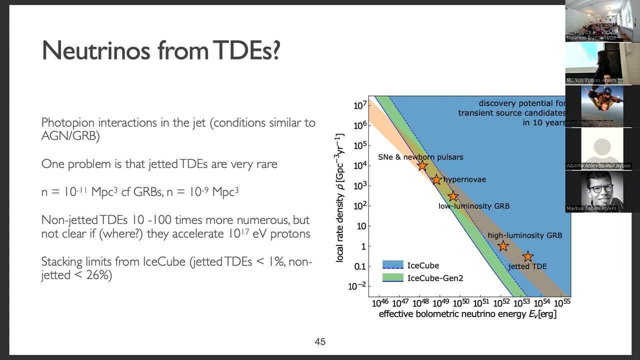 And because jetted tidal disruption events are very, very rare, they are constrained by this, by this non-detection of point sources And so stacking limits. also, an independent search for neutrinos from jetted tidal disruption events has put them to about no more than 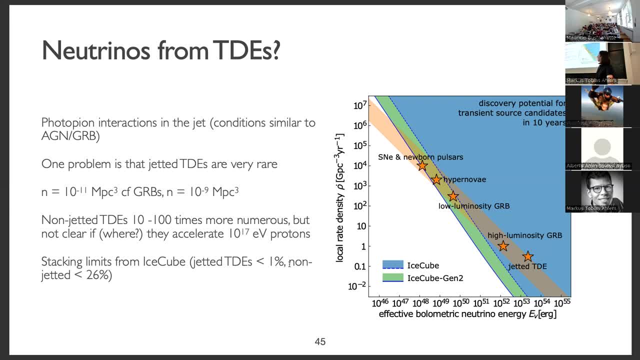 1% of the total neutrino flux. Now, only a small fraction of tidal disruption events have a jet. Those that don't have a jet are less constrained. They could make over there 30% of the total neutrino flux, But there there is no clear theory. where should 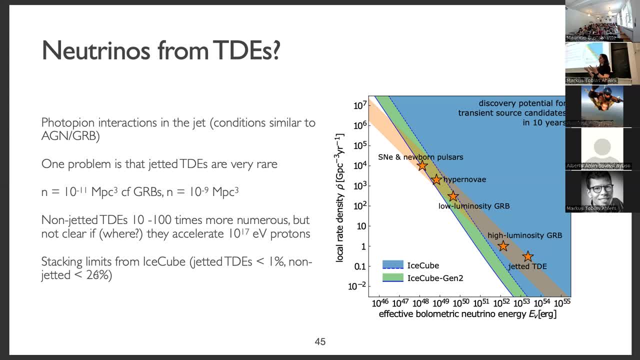 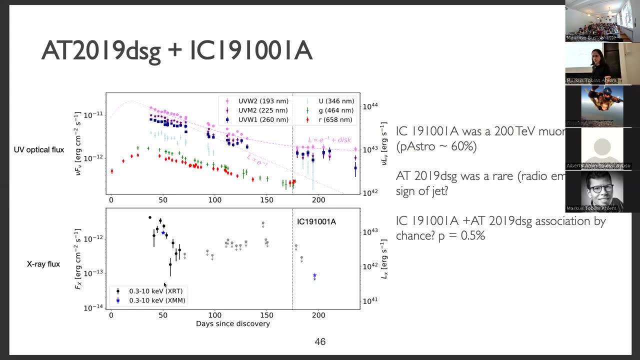 this acceleration of high-energy particles happen. Maybe you have something similar. we saw in non-jetted AGM before, something surrounding the accretion disk, but the theory is less well-developed In any case in 2019,. there was one neutrino. this is shown here. 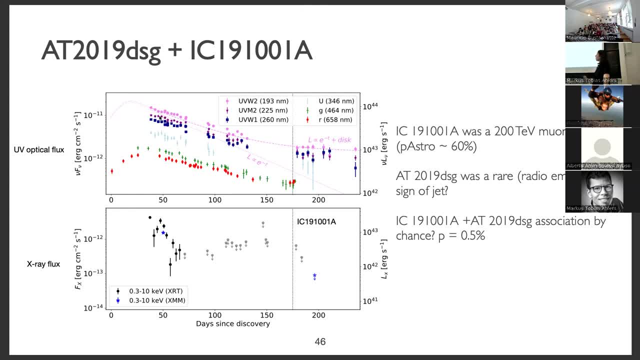 So this associated with one non-jetted tidal disruption events. So what's shown here is this decay of this tidal disruption event over 200 days. You see there is a peak and and then, within about 200 days, a neutrino was detected. 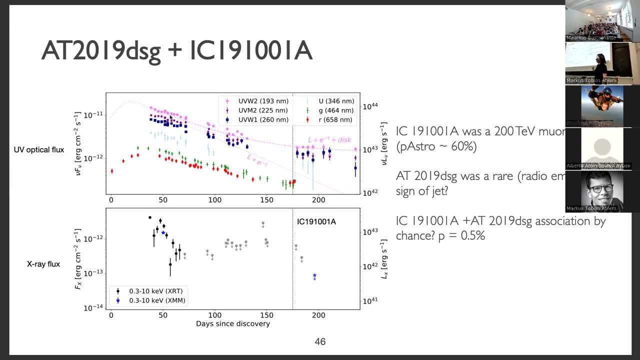 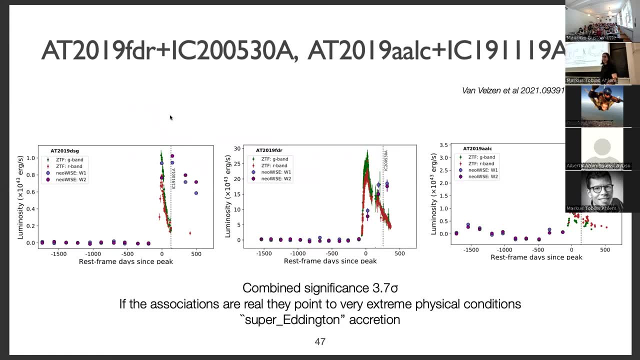 And the chance probability of such an event is 0.5%. And then, a year later, people- there was actually a few months later- there was a second event, Also the neutrino came within 200 days of the beginning of the. 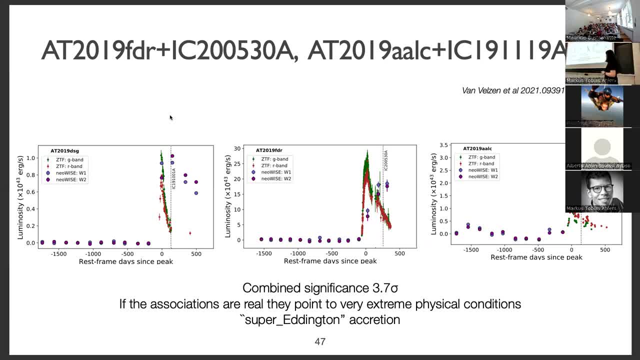 of the tidal disruption process. And then the people working on this looked at the archival ice cube data and found yet a third one. Now, this one is not confirmed as a tidal disruption event because it's in an AGM, But still the light curve looks like what you would expect. 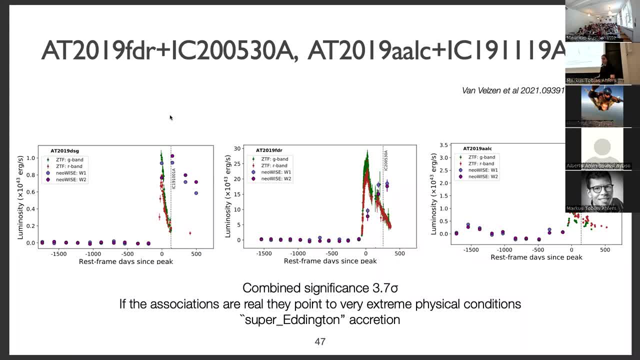 Also 200 days from the. I don't remember, maybe about 200 days from the time of the explosion. So now we have three. It's starting to get more interesting. The combined significance of all these three observations is the order: 3.7 sigma. 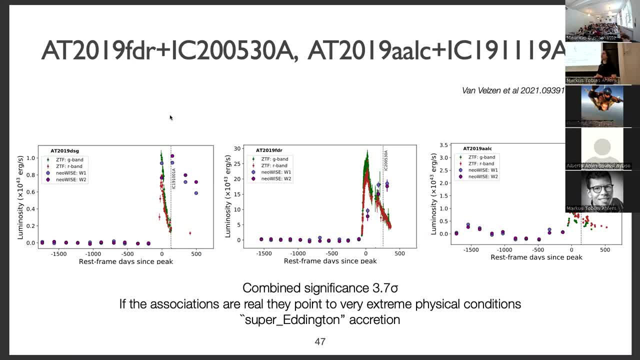 So you see, if we get the fourth and the fifth one, we will have to start to develop the theory better. But what I can say is that if all these are physical associations and not associations by chance, then the again we require a very extreme physical conditions in. 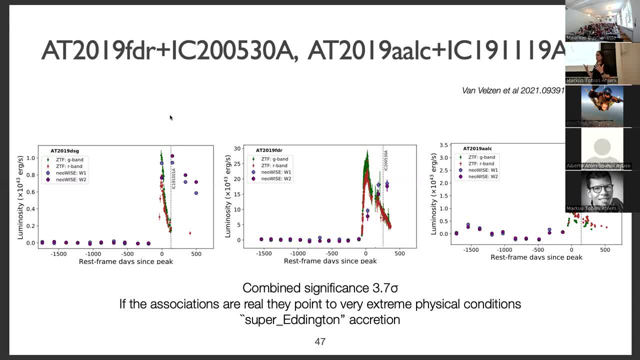 the sources, specifically super Eddington accretion, which is not something I'm heard of, but it just means some very extreme environments. So yeah, I would say they don't. if you see more of these, I would get excited. 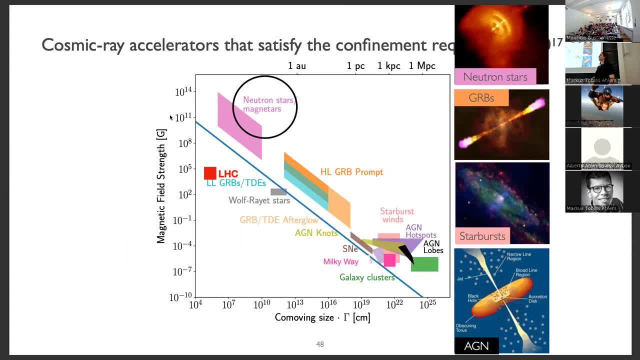 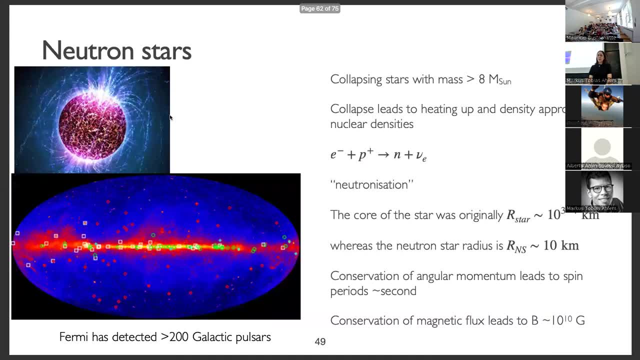 Final thing, neuter and stars. So I've been going down in in radius and up in magnetic field strength. So these here are, of course, what happens to a collapsing star with a relatively large initial mass, larger than eight times the mass of the sun, and in this process so we had the star which originally had. 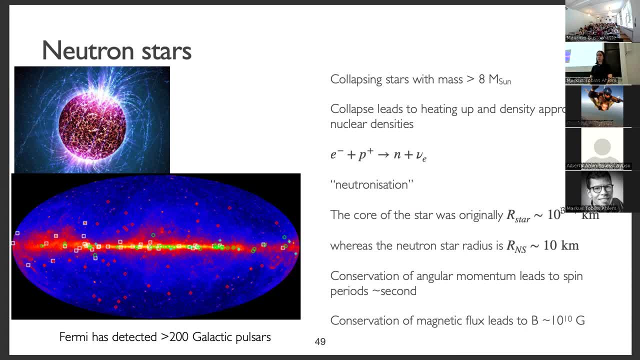 a radius of order ten to a thousand to ten to four kilometers, and it collapses down to ten kilometers, and so during this process we need to have conservation of angular momentum. this explains why they have extremely short spin periods of order seconds. we also have conservation of magnetic flux, so we start with something with a magnetic field like the sun and we end up with 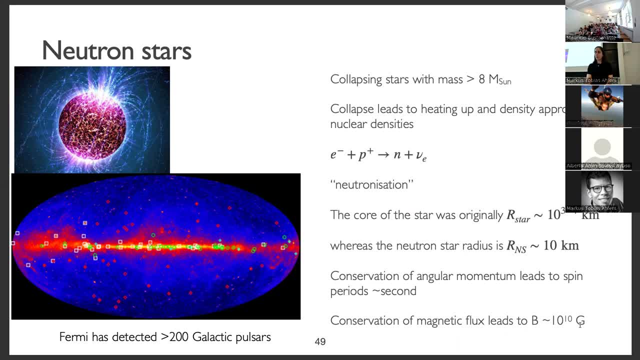 something with a magnetic field strength of order 10 to the 10 gauss, and there are several places in a neutron star where one can imagine acceleration of protons and neutrino production, either associated to the neutron star itself or associated with the wind, which we call the pulsar wind nebula, where we have astrophysical 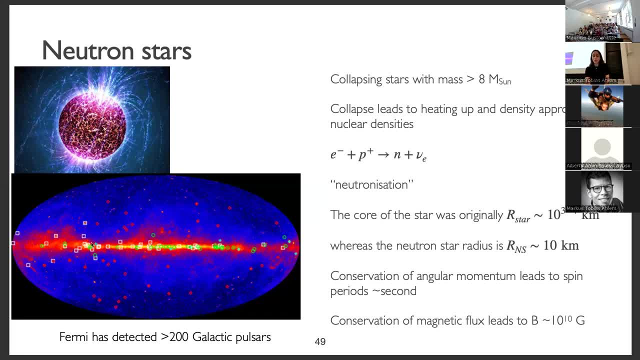 shocks. now fermi has detected of order 200 galactic pulsars. it means pulsars produce at least high energy electrons. here they are, these white squares in the figure, so they're all here in the galactic plane. and so if we were to ask ourselves whether 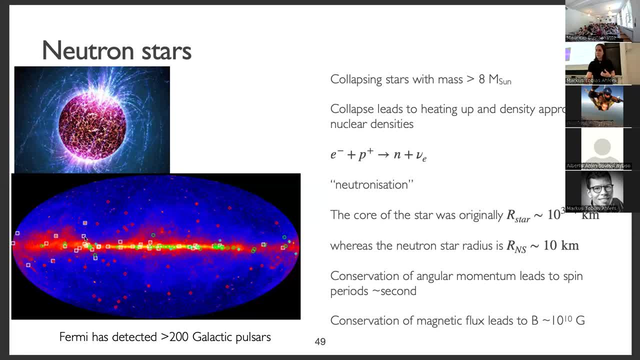 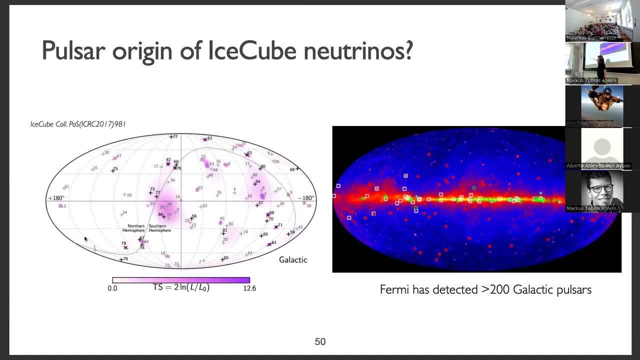 pulsars are consistent with producing the entire ice cube flux. then what i thought of is we can compare to the ice cube neutrino arrival directions and you see that there is no much excess of of galactic sources. so we we said there is an upper limit of the order of 15 percent of all neutrinos. 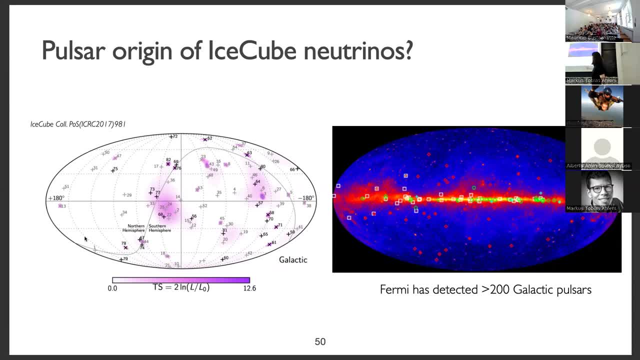 that could come from the galaxy, and i would say this is also the upper limit of. on galactic pulsars. if we invoke some special population of pulsars which is rare in our own galaxy, then we could have more, but galactic pulsars are constrained. yeah, yeah, yeah, i'm always bad, but which part of nuclear way can ice cube see and be seen by ice cube? 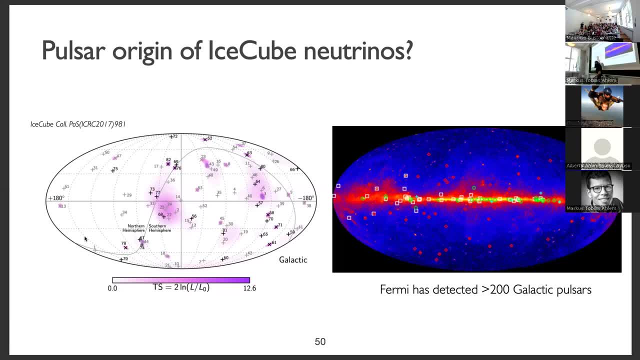 oh, good question. so you see here, here is the part that is nicely seen and it's the northern hemisphere, where the okay, eventually you have too much absorption in the earth and where all like, where are all pusherts located, okay? oh well, i'm not sure if this is the correct projection. some people, but okay, they should. 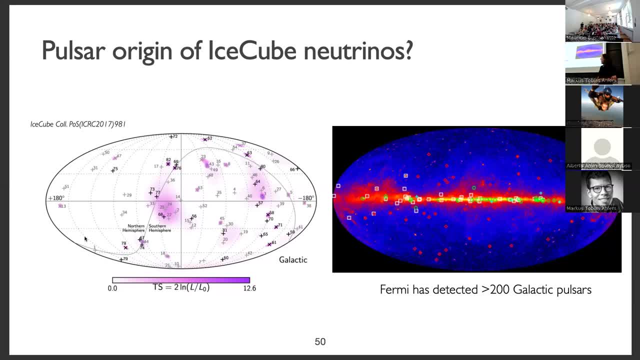 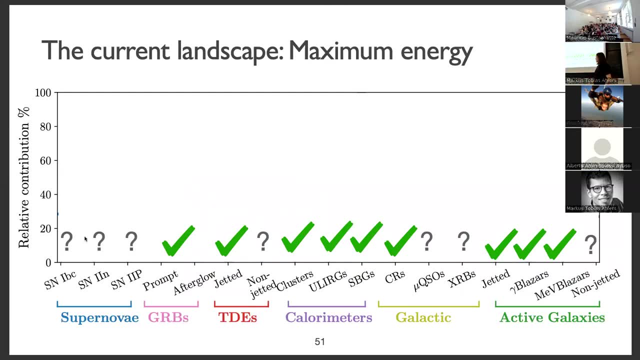 be on both sides. okay, yeah, okay, okay. so, um, this brings me to more or less the end of what i wanted to discuss. so i thought that what we could do at last is put everything we've discussed into one uh plot and start by saying: so i put here active galactic nuclei. 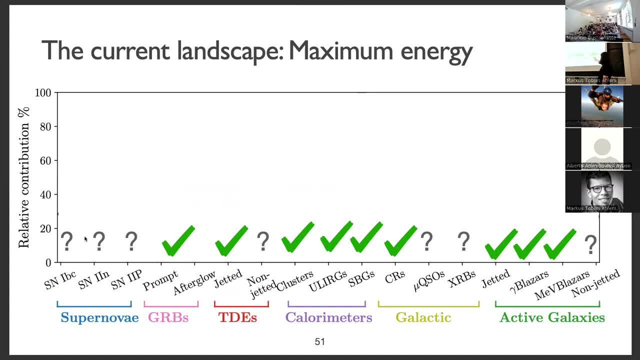 jetted agn gamma ray emitting blazars, non-jeted agn galactic sources like the cosmic rays. okay, these are, it doesn't matter, i didn't discuss these. these are micro quasars, calorimetric environments which are clusters of galaxies, starburst galaxies. 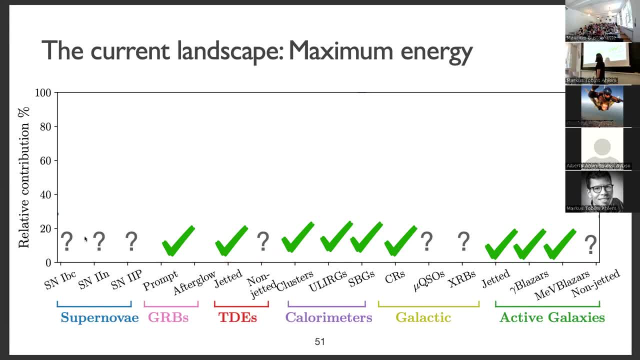 ultra luminous infrared galaxies, tidal disruption events, grbs and supernovae, which i didn't discuss much, but they could also produce high energy neutrinos. so the first requirement is that they should be able to accelerate sufficiently high enough energy particles. and here, okay, i've put in green all the sources. 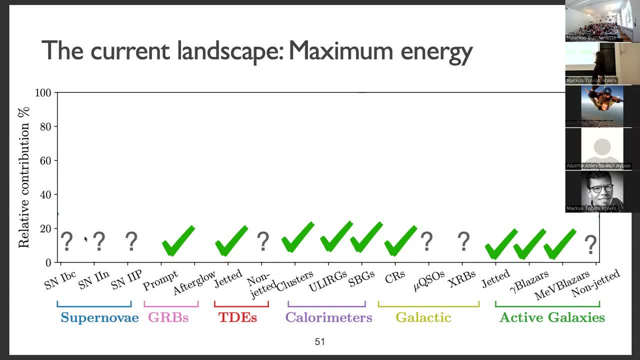 where they looked good in the hillas diagram and the rest i put with a question mark. i would say this is a kind of yes if it's a question mark. i mean we are not doing any extreme theory here, so we're just doing order of magnitude calculations. 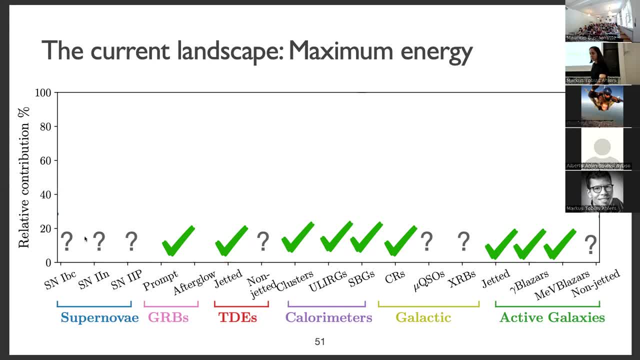 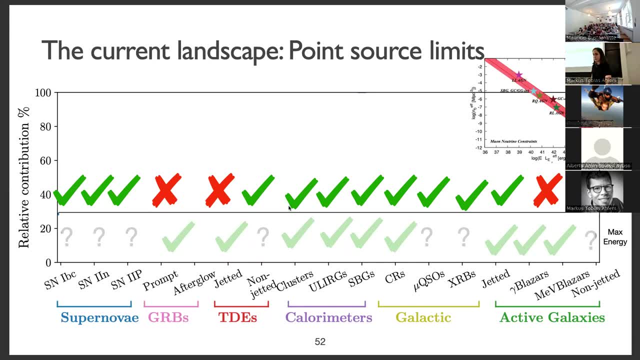 specifically supernovae, since I didn't discuss them there with the question mark. So now if we ask ourselves, do they satisfy the point source limit? constraint this idea that if they are very rare they would have already produced some point sources. you see what's left. 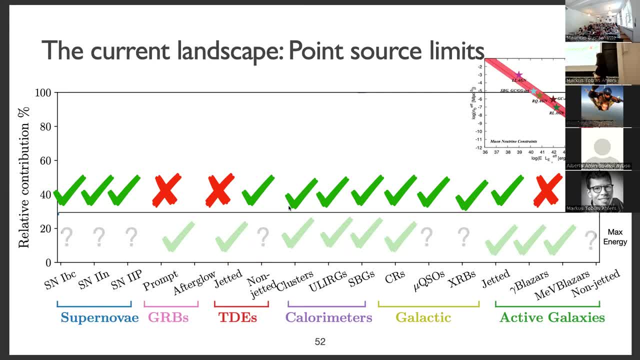 So actually what's interesting is what's left which ticks both boxes. so here I would say: non-jetted AGM are fine, starburst galaxies are fine. non-jetted tidal disruption events are fine and okay, supernovae are also fine. and then if we further ask ourselves if there is a connection to 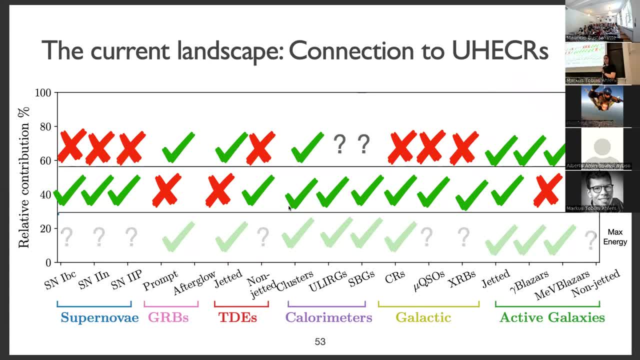 the ultra high energy cosmic resources. this is where things get bad. I couldn't find any which really work. maybe starburst galaxies, but they are themselves sort of challenging To produce ultra high energy cosmic rays themselves. but maybe there are transient explosions inside the starburst galaxies which could do it. 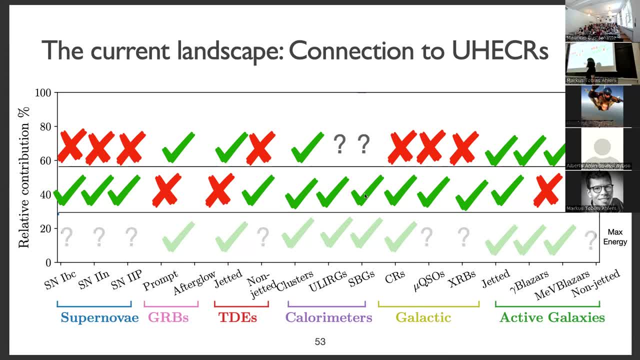 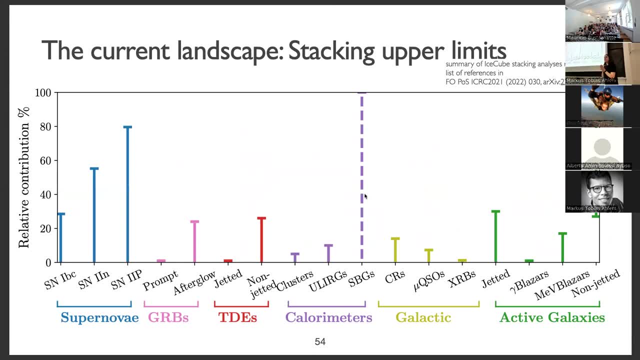 So you see that we're not left with many great candidates. I have here clusters of galaxies which are okay in all three, and now if I show you the upper limits from ice cube, from stacking searches on all of these objects, you will see that what's left is so most of these sources. 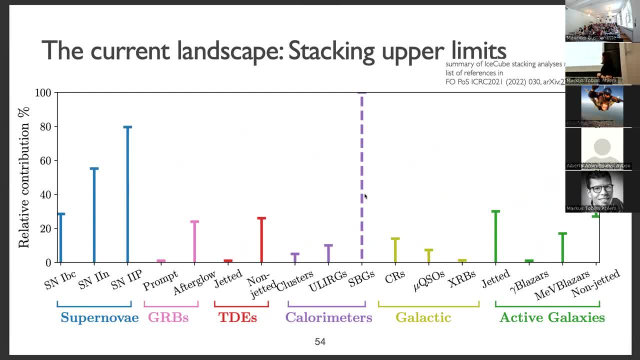 can produce at most 20 percent of the ice cube flux. Starburst galaxies are not constrained by stacking limits. supernovae- core collapse supernovae- are not well constrained and the jetted AGM- this is the result of this study that I showed- are also okay, But somehow none of them are the. 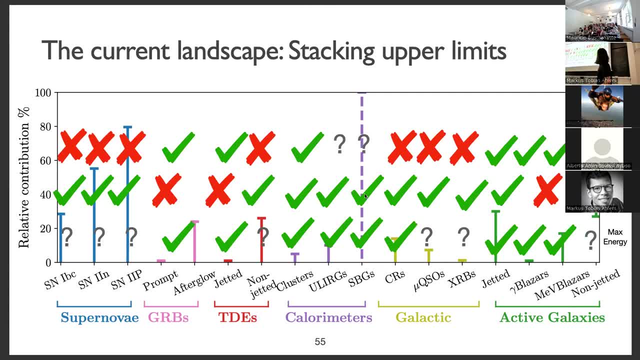 populations. one might have guessed. so if I put them all together, they are not necessarily the most obvious candidates. This doesn't mean that all these other sources don't produce neutrinos, and I didn't have time to talk about it. but we have another energy range, above the ice cube energy range, where we expect. 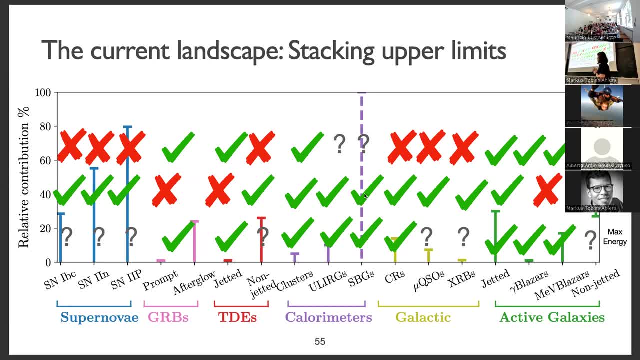 a lot of new detectors which might look for the neutrinos which connect better to the ultra high energy cosmic rays. I also want to say that there is the fact that these are not very rare, like starburst galaxies or core collapse. supernovae in the whole universe is why we can't constrain them, so we can better constrain sources which are 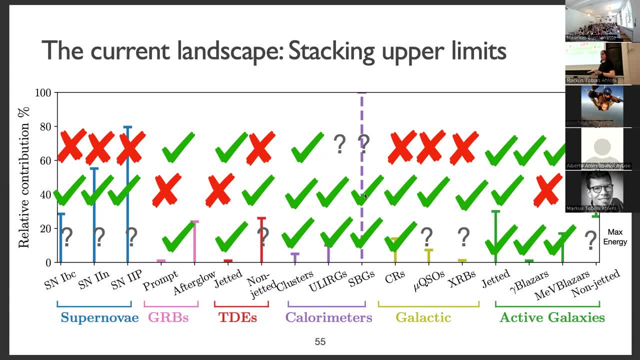 rare because we can stack them more efficiently. And so, yeah, I mean some of these you could turn. how should I say? this is only a hand waving way to classify all these, and I encourage you to go into the details of the theory to find your own answers to all this. and with this I'd like to stop and thank you very much. 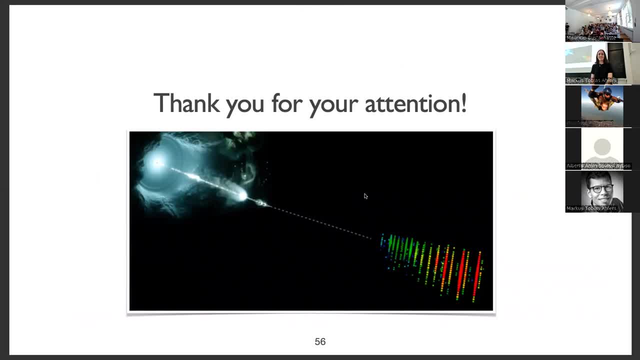 Thank you, Fotini, for today and also the lectures that you delivered on Monday. Other questions, Hi. one thing we assume all the time is that the branching ratio is of the protons is around one right. isn't that at all dependent on the medium where? 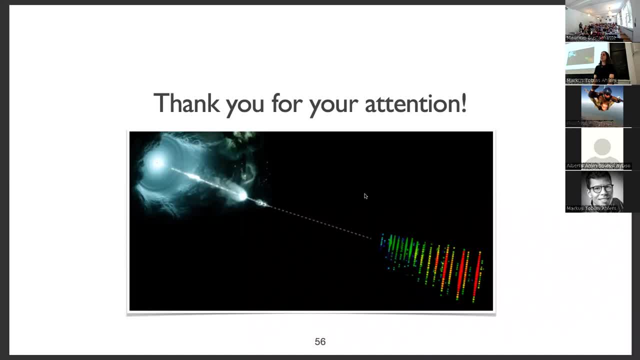 where the proton? well, where the pion? well, which pion will be, yeah, created? Are you saying that we are assuming the the neutral to charge pion branching ratio is about one? Yes, yes, Yeah, okay, I am not aware of any reason why this could be severely modified. 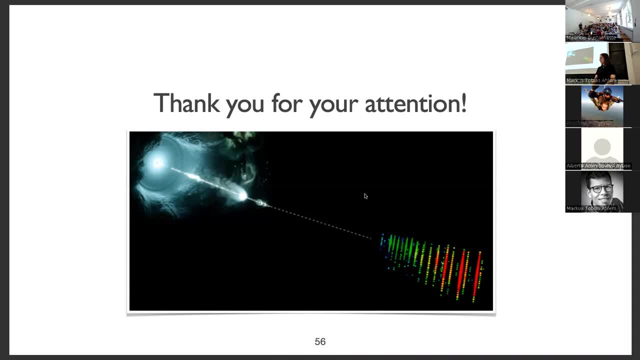 in photopion interaction. so I don't know. Mauricio is not here, Markus, do you? I don't know either, but that was just something. maybe there's some. I think so actually. I mean, these are, of course, like ultra-energy, cosmic rays, but if you calculate the center of mass energies, this is just. 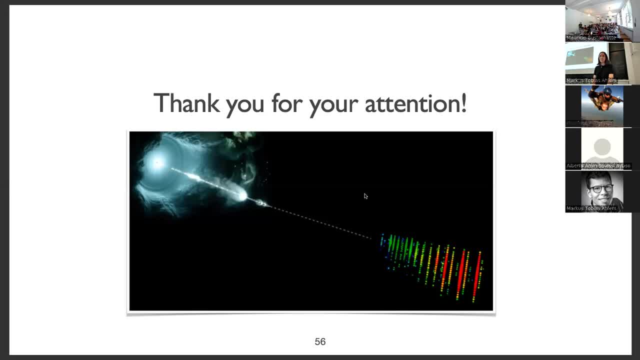 lab energy. so this is actually fairly well covered in lab experiments. so we know the pion multiplicity there very well. so it depends a bit on p-t and p-gamma interaction, but it's always roughly at the same order of magnitude. yeah, I'm not sure who was first. 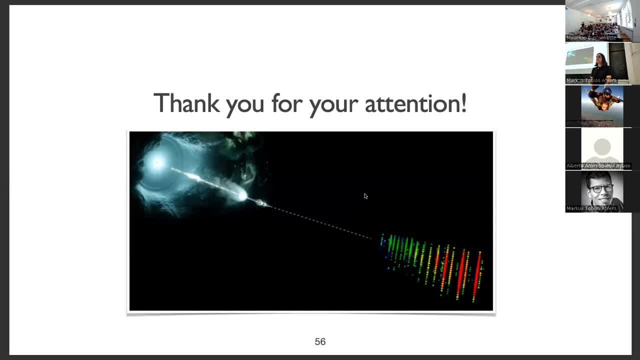 Okay, thanks, Um, uh, just to get this right about the gamma ray burst. so they come in two families: one is very short, one is a little bit longer. and do we think now that all the short ones come from neutron star mergers? Yes, Okay, because we saw, uh, in this neutron star merger where we got a gravitational waveform then there, 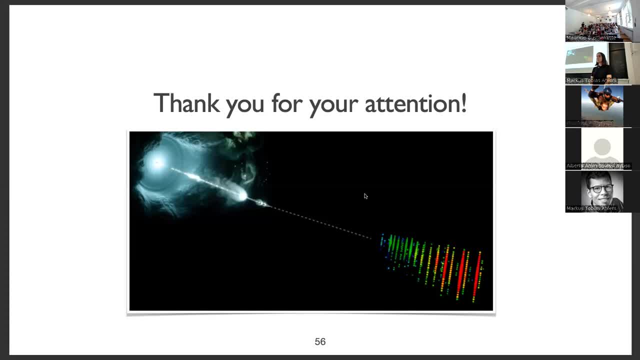 we saw that one was really short and this would explain that there's this gap between the short ones and the longer ones. Is this the The reason why we can be sure- So it was theoretically predicted long ago that there is- that the long ones come from the death? 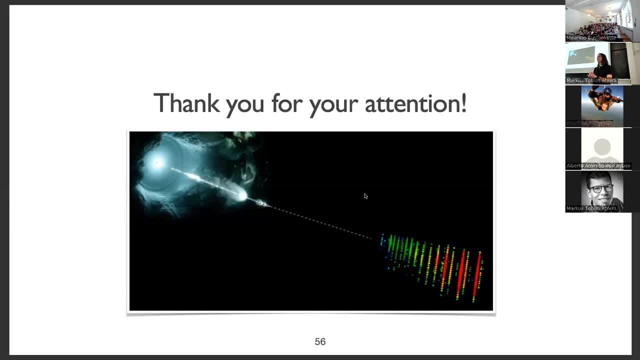 of a single massive star and the short ones come from this neutron star merger and we had small indirect evidence in this direction. for example, short grbs happened only in environments where we expected, like only in galaxies where we expected there to be lots of neutrons. 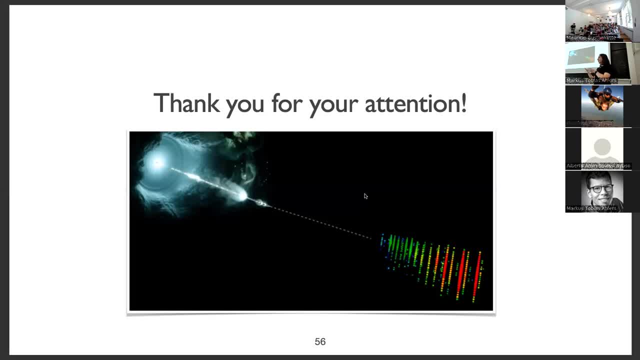 Star binaries, and long ones, happened preferentially in places where we expected them to be enriched in massive, uh, in massive stars. so this was just the final thing we needed to confirm the origin of the short grbs. um, and yeah, Okay, great, Uh, my question is a little more general. uh, so what are the expectations, or your expectations, for the? 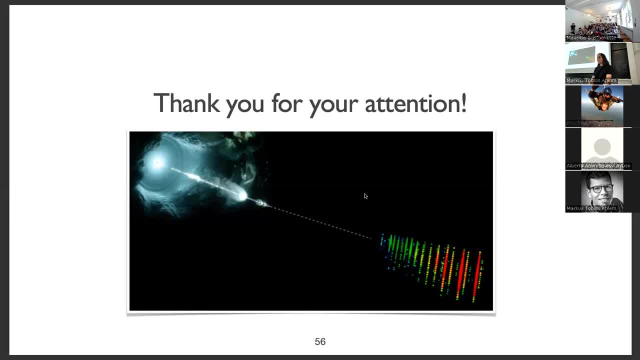 field in the next uh 10 years. So you have shown us a lot of uh this study. there are a lot of sources for neutrinos and there are some constraints, and how would the field will evolve for these next 10 years? what are the expectations? 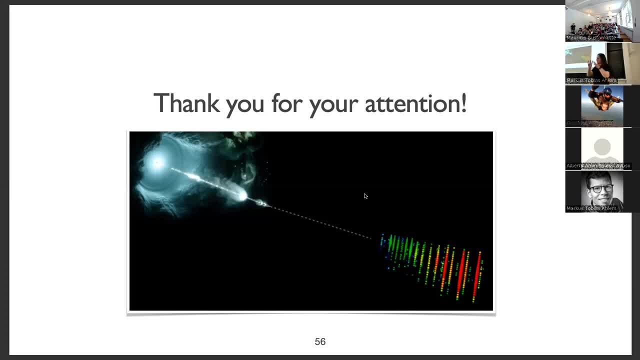 Yeah, thank you. this is such a great and general, like big question. um, I think progress is going to be slow because we are only detecting neutrinos at this rate until we have ice cube gen 2, which will be a size 10 times, or not exactly 10 times, maybe five times, six times larger. 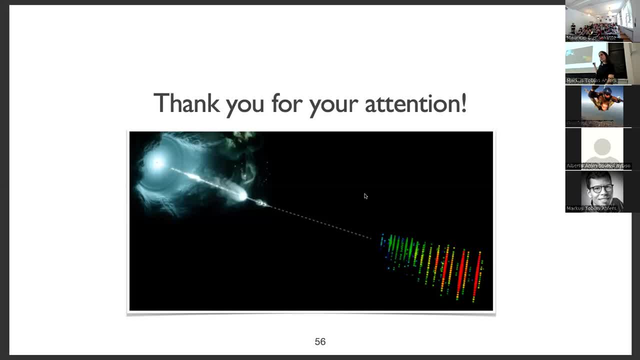 We have seen that it's easier to constrain a source class than to confirm it. so I expect the, the stacking limits to become- uh, you know, just to continue to, to, to increase in significance and, as, as marcus told us, if we expect the success to grow, 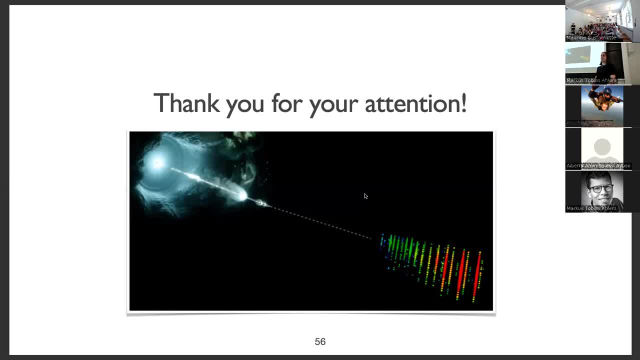 for a particular population, we need at least to double the observation time. Now what's happening is we have optical surveys which will be much more sensitive than today's ones. so we're going to have a lot of optical transients, for example, associated with each neutrino, so the theorists will have a lot more work to model all of them and say which one. 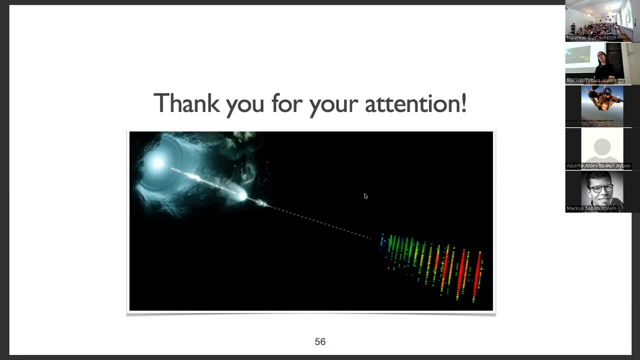 um, So we will have more false positive associations, and so we'll have a lot of modeling work to do to say which one of these sources is plausible and which one isn't. So we'll have a lot of papers and the archive and a lot of activity. Yeah, that's my expectation. Okay, thank you. 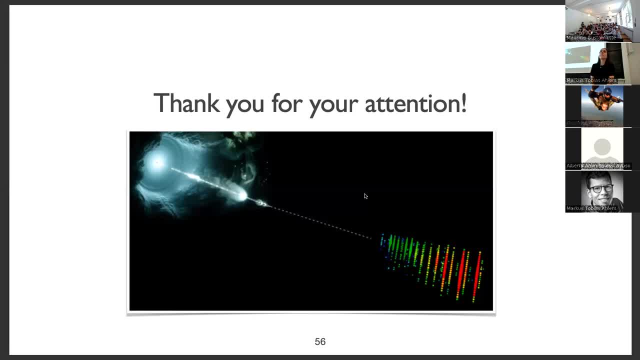 So my question is about the magnetic field in neutron stars. You said it's 10 to the 10 goals, So I think that if you have a neutron star merger, I think this magnetic field increases by a lot, right Decreases. It increases in neutron star merger. Well, so one doesn't really know what happens when you have a neutron star merger and what is the final object. I don't know if this is more, if this is what your question is. Yeah, no, it's because I read that in neutron stars. 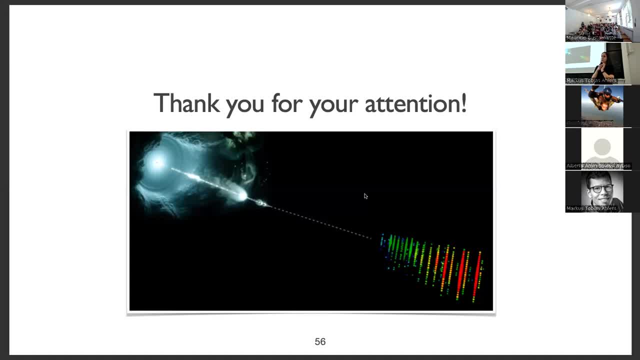 it's expected that the magnetic field reach like 10 to the 16 goals. Okay, I think so. That's a general. All neutrons, That's a general. stars, it doesn't matter if they are merging or not. they sort of spin down in time and their 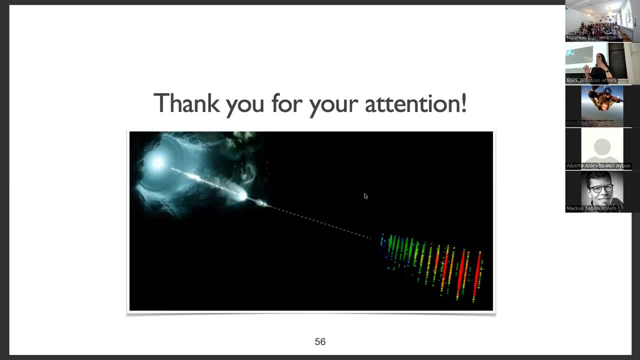 magnetic field also sort of is dissipated in time. so they start off very magnetized and that drops off this time. okay, so as you said, to increase the neutrino production, we can increase the number of injected proton. so then, what about the eddington limit in that case? so yes, thanks for this question. so 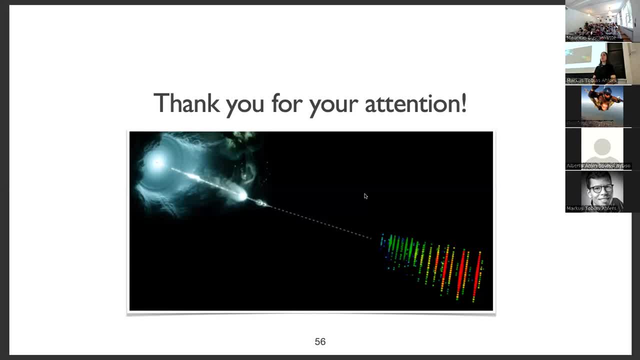 i am not aware of any model in which we can have super eddington accretion in supermassive black holes. there are a lot of problems that then happen to the galaxy, like too much feedback and you stop the star formation and so on. the models that i showed for texas 0506. 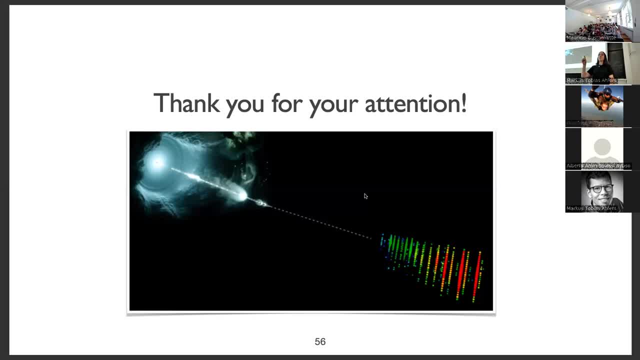 require super eddington proton luminosity. so this is a problem. how did that happen in this source? and maybe it can happen for a short time, but if it were to happen for a long time, we have all kinds of problems within, even with galaxy evolution. so this is a 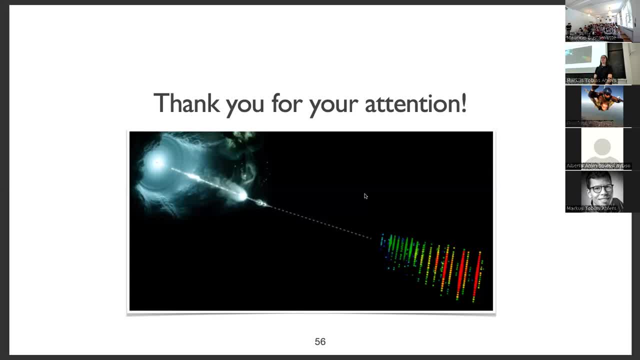 nobody knows if this happens or not. in aegean you also had starburst galaxies on your summary slide. there there's also some correlation of alpha energy cosmic rays with starburst galaxies. this is true, this is true, this is true. yeah, actually, i think starburst galaxy is so far too. 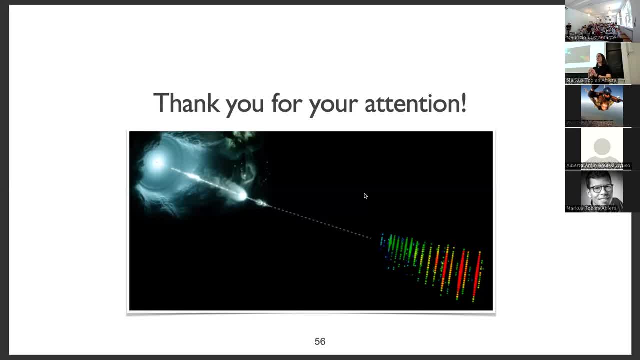 far away from the starburst galaxy. but i think everything is so far away from the starburst galaxy. so, yeah, what marcus refers to is that if we look at the arrival directions of all the ultra high energy cosmic rays, they are deflected, so they're not as perfect as neutrinos. but then we have a. 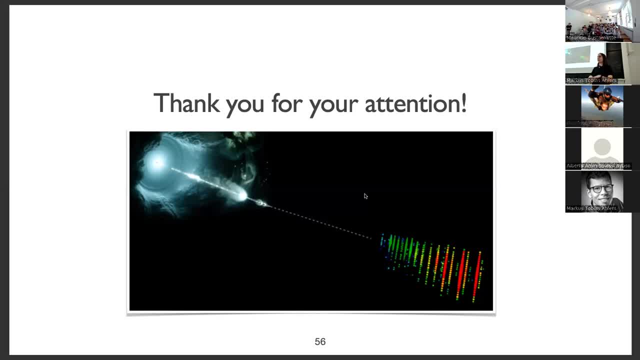 four, point. four point: something sigma excess of cosmic rays from starburst galaxies than we would expect from background. so this is interesting. yeah, one last question, since you are talking about the ice cube, gen 2. so how is it going to enlighten in future about our learning on the combination of different cosmic messengers?